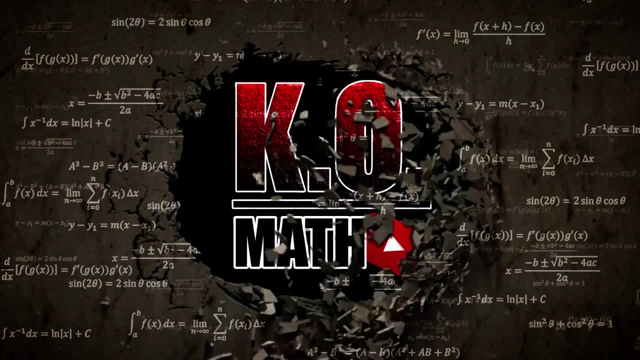 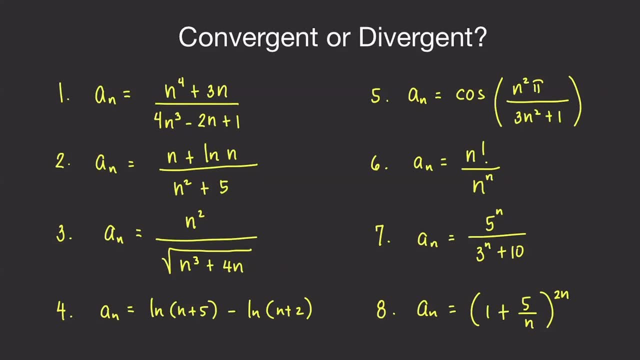 In this video we're going to discuss convergence and divergence of sequences. In particular, we're going to show the convergence or divergence of the following sequences: So a sub n denotes the nth term of a given sequence. Let's get started. So let's look at this first sequence here, where 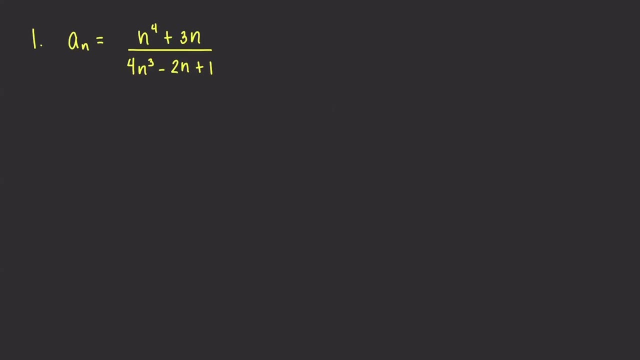 a sub n is equal to n raised to 4 plus a 3n, all over 4n cubed minus 2n plus 1.. Recall that to show that a sequence is convergence. we need to show that the limit of a sub n as n goes to infinity. 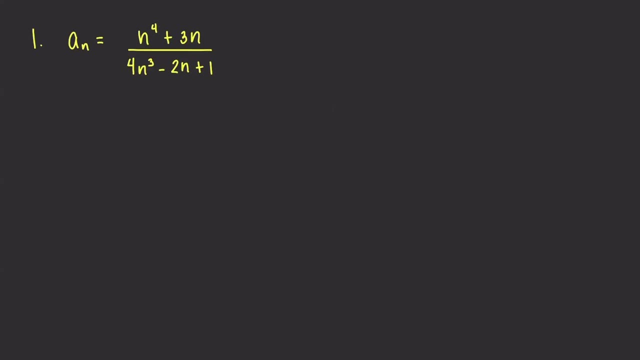 exists, which means it's a real number. If the limit does not exist, then we say that the sequence is divergent. So let's compute for the limit of a sub n as n goes to infinity, which is equal to the limit, as n goes to infinity, of n raised to 4 plus 3n over 4n cubed minus 2n plus 1.. 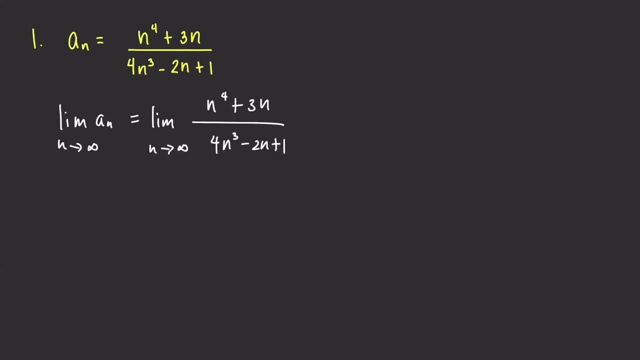 So this is similar to computing limits of rational functions. So as n goes to infinity, this goes to infinity, this goes to infinity. But our technique when we're computing limits of a rational function at infinity is to divide the numerator. So we just run the numerator and denominator by the highest degree term in the denominator. 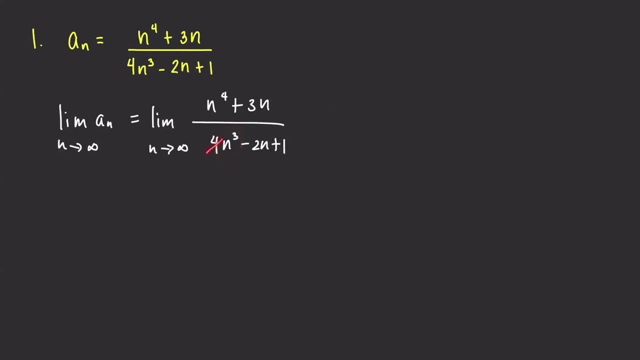 excluding the constant. So you may exclude this coefficient here, which is equal to four. So we just have to divide the numerator and denominator by this highest power of n in the denominator, which is equal to n cubed. So here we have limit, as n goes to infinity. So thepara is the letter of the denominator and numerator is equal to minus 4 by the numerator. So if our 정init etc is h1 all over 4, we can compute that in the denominator. So we have to provide data back like a form and then we can calculate the numerator. Can you give a definition? if the denominator is this, Do we have other things like the denominator is this? So let's go into this. Let's do the definition associated with norm numerator, numerator denominator properties. 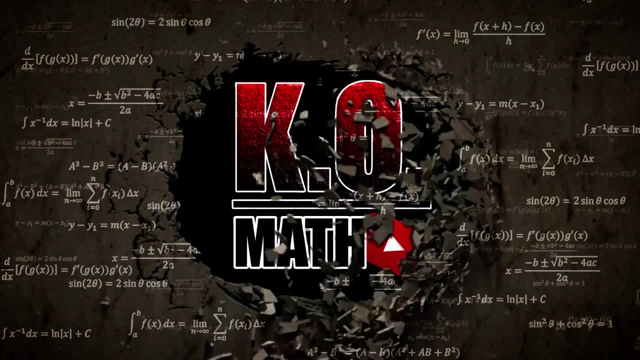 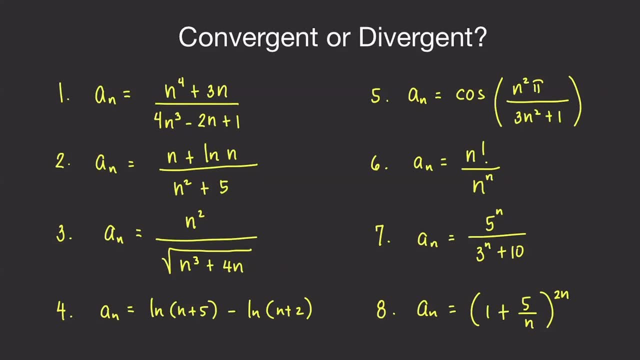 In this video we're going to discuss convergence and divergence of sequences. In particular, we're going to show the convergence or divergence of the following sequences: So a sub n denotes the nth term of a given sequence. Let's get started. So let's look at this first sequence here, where 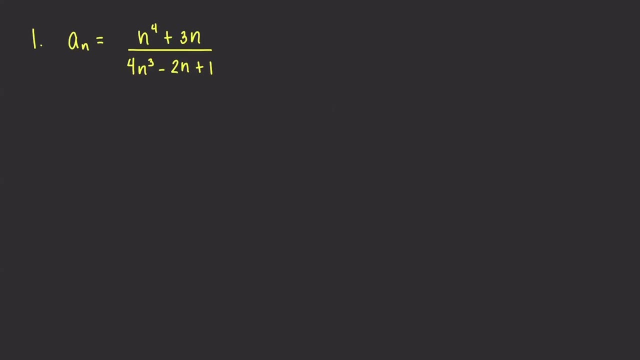 a sub n is equal to n raised to 4 plus a 3n, all over 4n cubed minus 2n plus 1.. Recall that to show that a sequence is convergence. we need to show that the limit of a sub n as n goes to infinity. 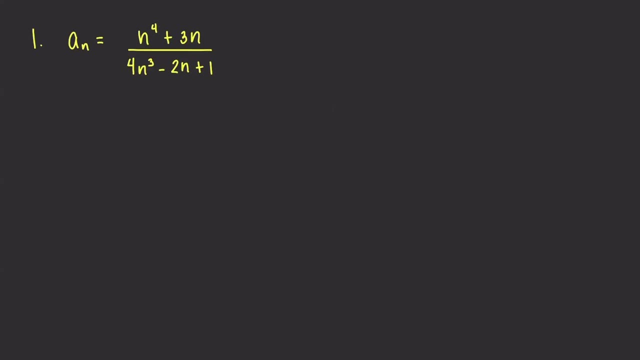 exists, which means it's a real number. If the limit does not exist, then we say that the sequence is divergent. So let's compute for the limit of a sub n as n goes to infinity, which is equal to the limit, as n goes to infinity, of n raised to 4 plus 3n over 4n cubed minus 2n plus 1.. 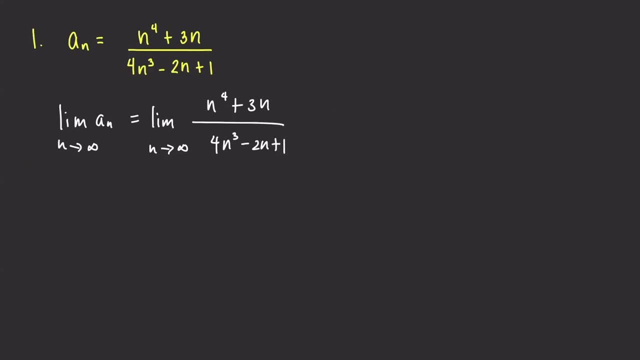 So this is similar to computing limits of rational functions. So as n goes to infinity, this goes to infinity, this goes to infinity. But our technique, when we're computing limits of a rational function at infinity, is to divide the numerator and denominator by the highest degree term in the denominator, excluding the. 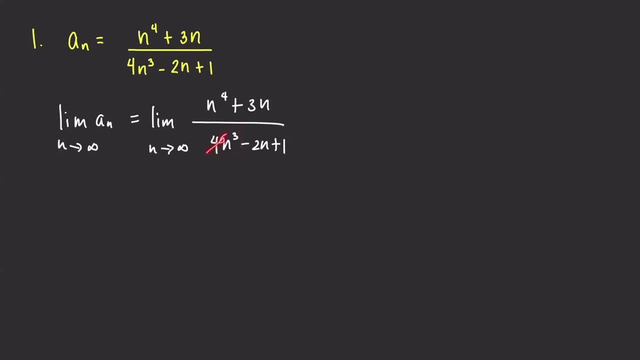 constant. So you may exclude this coefficient here, which is equal to 4.. So we just have to divide the numerator and denominator by this highest power of n in the denominator, which is equal to n cubed. So here we have limit, as n goes to infinity. 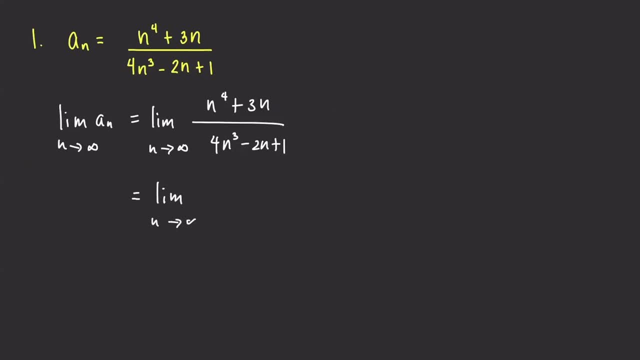 So we have a difference of � nuances divided by a number in terms of intuition with respect to a conditions. infinity of n raised to 4 you divide this by n cube and then also the numerator you have here a 3n over n cube and then over 4 n cube over n cube and 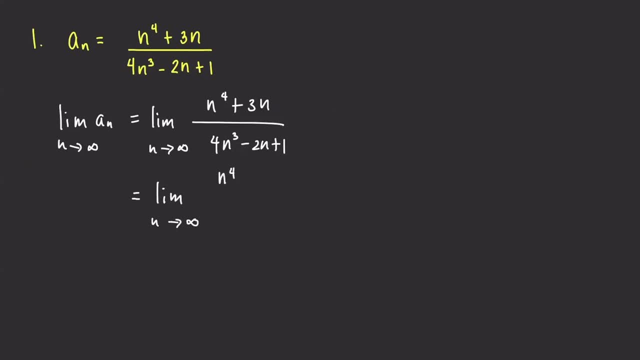 n goes to infinity of n raised to 4. you divide this by n cube and then also the numerator. you have here 3n over n cube and then over 4n cube over n cube, and then minus 2n all over n cube and then plus 1 over n cube, and when we simplify this fraction we get n minus 3 over n squared. 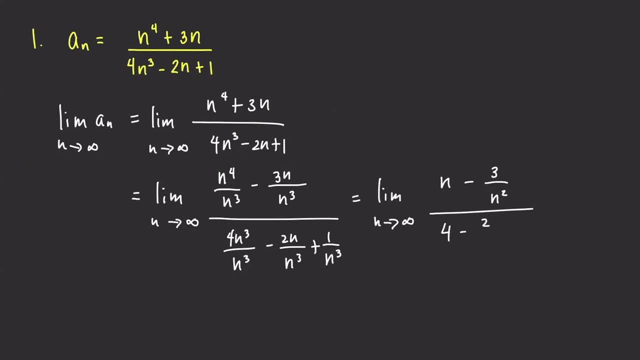 over. you have here 4 minus 2 over n squared, and then plus 1 over n cube, and the limit, as n goes to infinity in this case, is equal to. so this goes to zero, this goes to zero, and then this term also goes to zero. so, as you can see, here our numerator goes to. okay, this one. 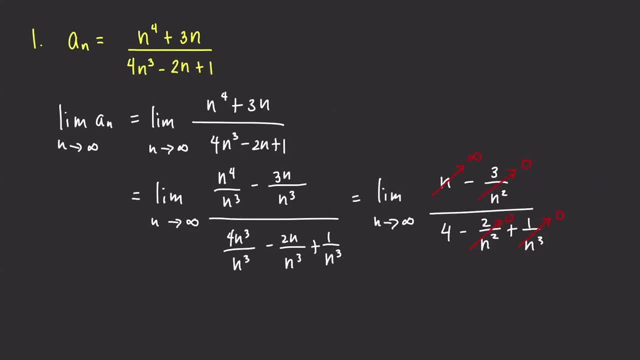 goes to infinity. so the numerator goes to infinity and the denominator goes to 4. so therefore the limit of this sequence is equal to infinity. so therefore the sequence a sub n is divergent. now let's move to the next problem. here we're given a sub n equal to n plus l and n all over. 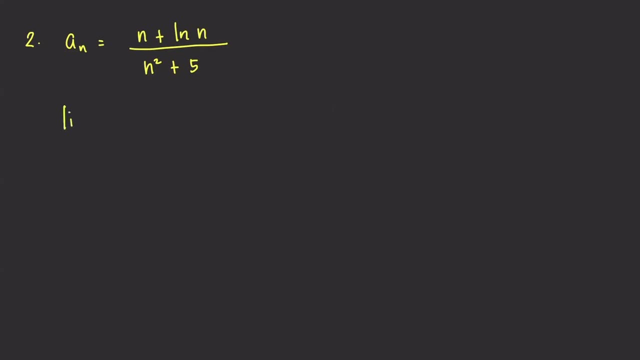 n squared plus 5, so we compete for the limit. so limit of a sub n as n goes to infinity, which is equal to limit of n plus l and n all over n squared plus 5, so we compete for the limit of 5. so part of the rule is now that we have n plus 1 squared plus 5, as n goes to infinity. 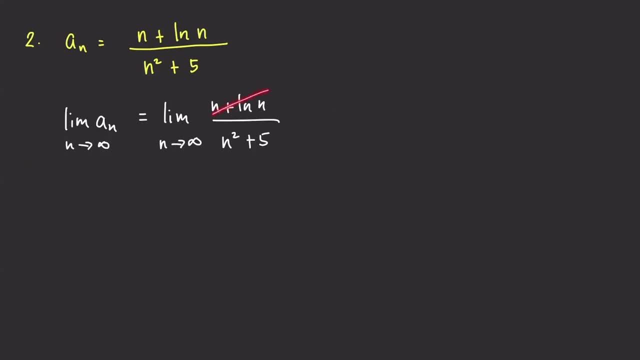 now, as n goes to infinity, the numerator goes to infinity and also the denominator goes to infinity. so we have a limit of the form: infinity over infinity. and if we have such a limit, so we may apply l-hop. but for l-hospital's rule we need to take alh�pital's rule. but for alh�pital's 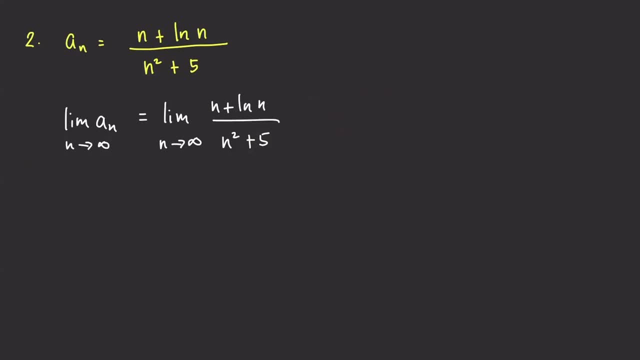 we need to compute for derivatives. but keep in mind here that the values of n are just the integers. okay, so that we can apply el hospital's rule. there's also a theorem that we could use here, wherein this limit is just equal to replacing the n by a continuous variable. 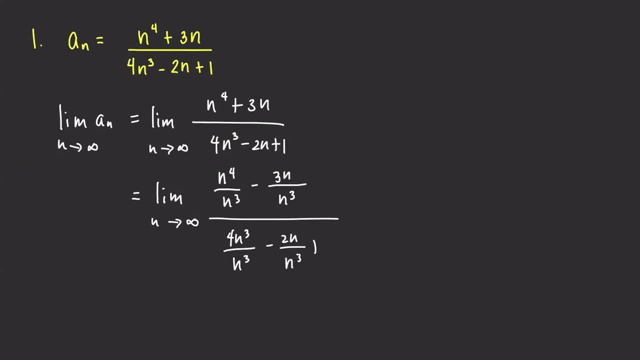 then minus 2n all over n cube, and then plus 1 over n cube, and when we simplify this fraction we get n minus 3 over n squared over. you have here 4 minus 2 over n squared, and then plus 1 over n cube, and the limit as n goes to infinity. 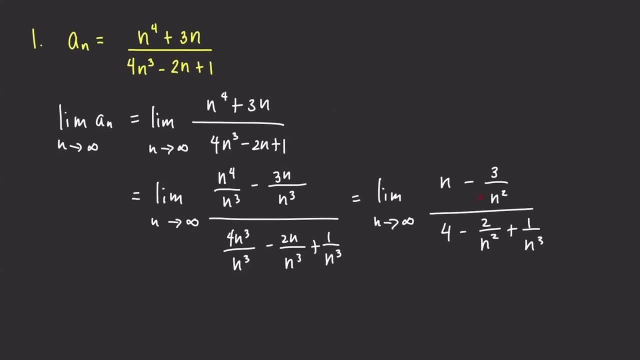 in this case, is equal to. so this goes to 0, this goes to 0, and then this term also goes to 0. so, as you can see, here our numerator goes to okay, this one goes to infinity. so the numerator goes to infinity and the denominator goes to 4. so therefore, the limit of this 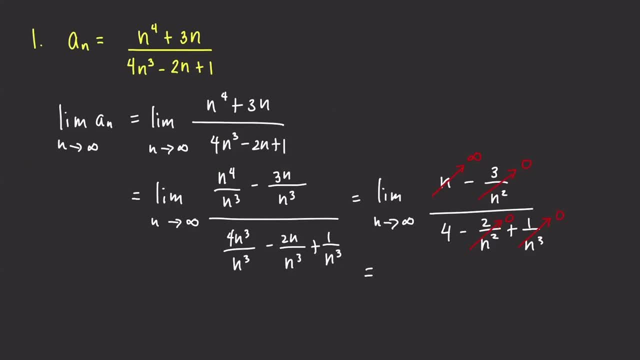 sequence is equal to infinity. so therefore the sequence a sub n is divergent. now let's move to the next part problem. here we're given a sub n equal to n plus ln, n, all over n squared plus 5. so we compete for the limit. so limit of a sub n, as n goes to infinity, which is 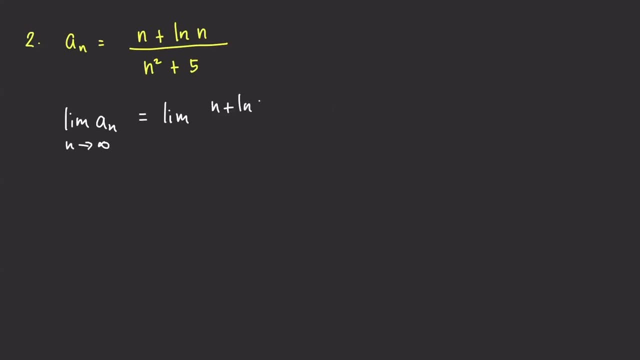 equal to limit of n plus ln, n all over n squared plus 5, as n goes to infinity. now, as n goes to infinity, the numerator goes to infinity and also the denominator goes to infinity. so we have a limit of the form: infinity over infinity. and if 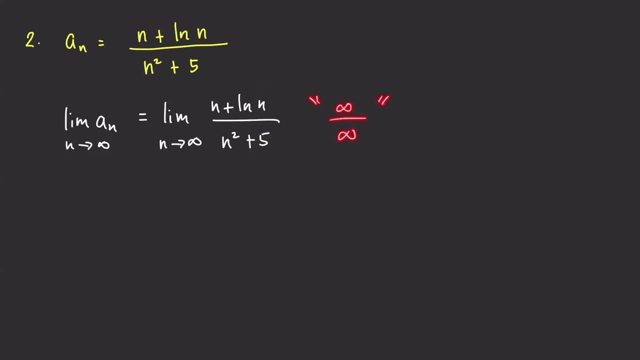 we have such a limit, so we may apply L Hopital's rule. but for L Hopital's rule we need to compete for derivatives. but keep in mind here that the values of n are just integers. okay, so that we can apply el hopital's rule. there's also a theorem that we 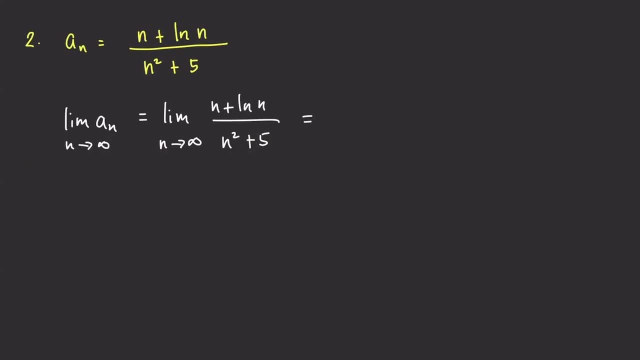 could use here, wherein this limit is just equal to replacing the n by a continuous variable. x goes to infinity. okay, it is just equal to x plus l and x and then all over x squared plus five. so the reason we change the variable here is is that so that we can apply el hopital's rule. 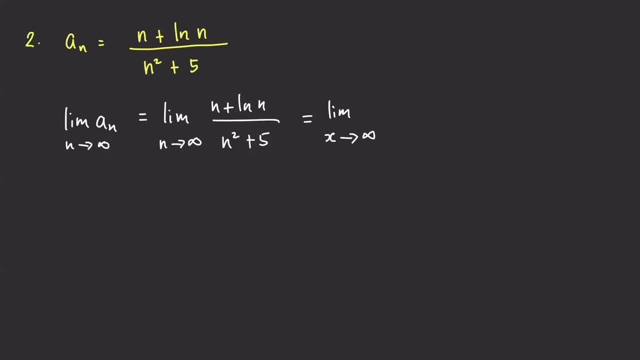 x goes to infinity. okay, it is just equal to x plus l and x and then all over x squared plus five. so the reason we change the variable here is that so that we can apply el hospital's rule, because el hospital's rule we have to compute for the derivative and we need, if you're considering, 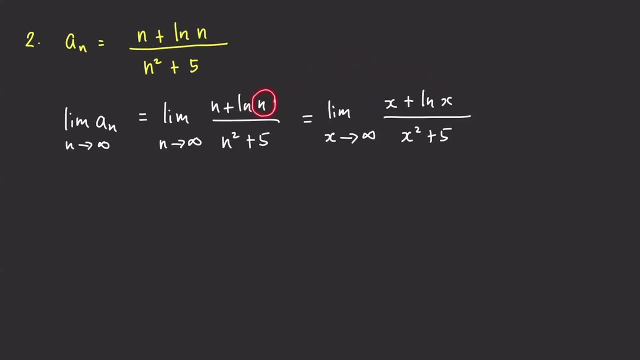 only discrete values of x, then for sure it is not differentiable at any point. so it is not differentiable at one, at two, three and so on. we'll get here, since this is an indeterminate form, indeterminate form, infinity over infinity. so we can apply now. 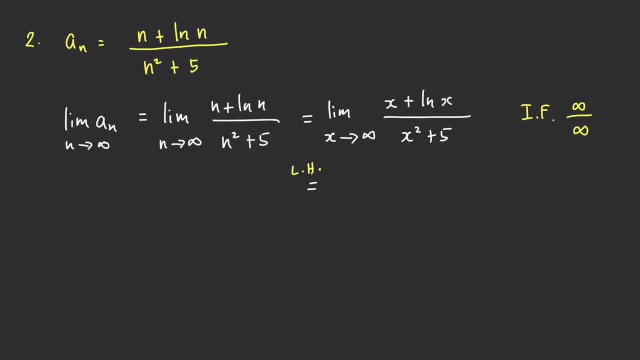 el hospital's rule. so this is equal to limit, as x goes to infinity, of derivative of the numerators, that is, one plus one over x and then over the derivative of the denominator, which is equal to two x, as x goes to infinity. all right, so as x goes to infinity, in this case, it is clear that our denominator here goes to. 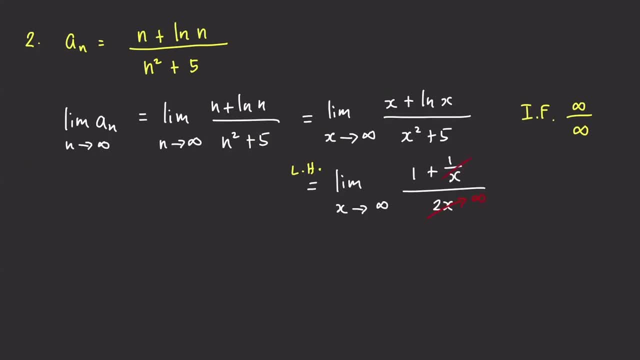 infinity, and this one over x goes to zero. so, as you can see from here, we have a limit which is in the form. this is in the form: one over infinity, so one over a huge number, so that is what a very small number. so the values of this are getting closer and closer to zero. so therefore, 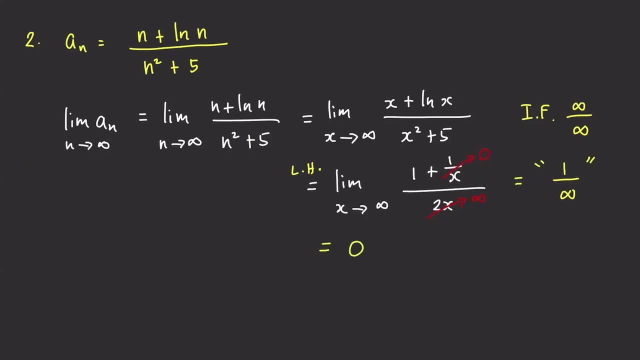 the limit of this one is equal to zero, since the limit exists. so therefore the sequence a sub n is convergent. let's move to the next problem. so we have here a sub n which is equal to n squared over squared of n cube plus 4n. so again we use the same idea in finding limits of a rational function. okay as n. 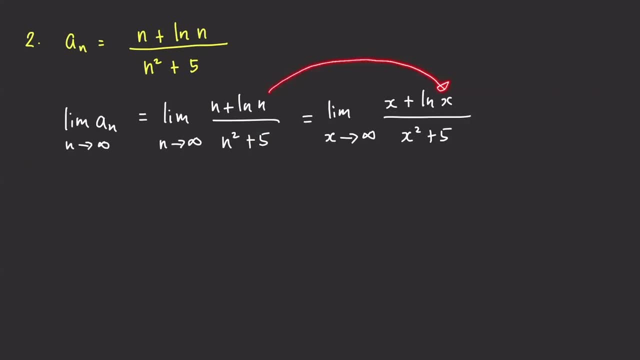 because el hopital's rule: we have to compute for the derivative and we need. if you're considering only discrete values of x, then for sure it is not differentiable at any point. so it is not differentiable at one, at two, three and so on. we'll get here, since this is an indeterminate form. 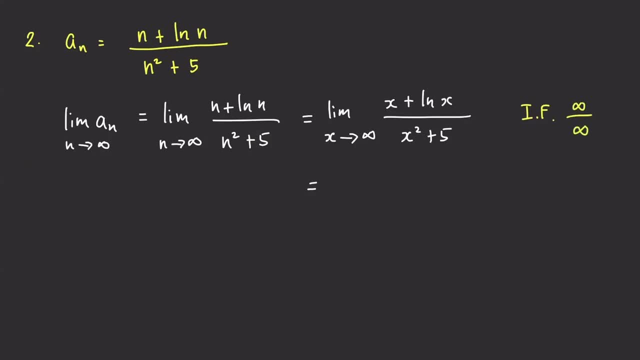 indeterminate form, infinity over infinity. so we can apply now el hopital's rule. so this is equal to limit, as x goes to infinity, of derivative of the numerators, that is, one plus one over x, and then over the derivative of the denominator, which is equal to two x as x goes to infinity. 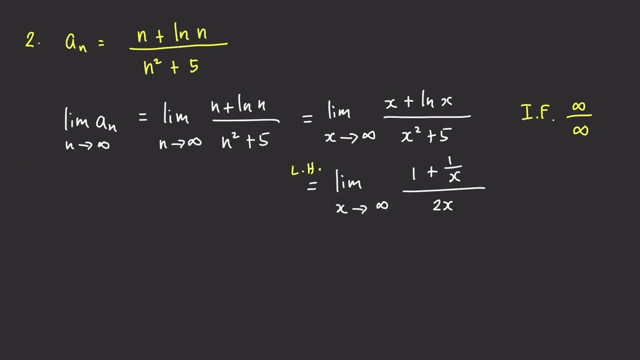 all right. so as x goes to infinity, in this case it is clear that our denominator here goes to infinity and this one over x goes to zero. so, as you can see from here we have a limit which is in the form. this is in the form: one over infinity, so one over a huge number. so that is what a very 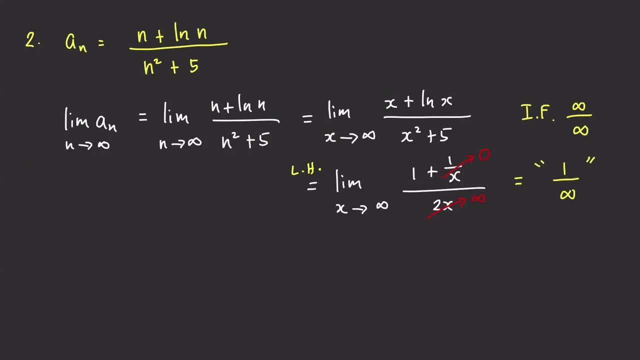 small number. so the values of this are getting closer and closer to zero. so therefore the limit of this one is equal to zero, since the limit exists. so therefore the sequence a sub n is convergent. let's move to the next problem. so we have here a sub n. 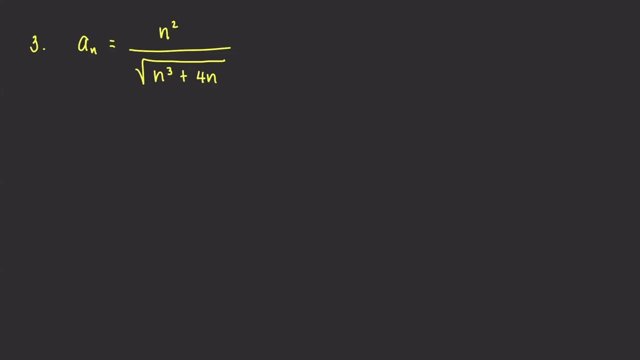 which is equal to n squared over square root of n cube plus four n. so again we use the same idea in finding limits of a rational function. okay, as n goes to infinity, it's like dividing the numerator and denominator by the highest power of n in the denominator. but since we have 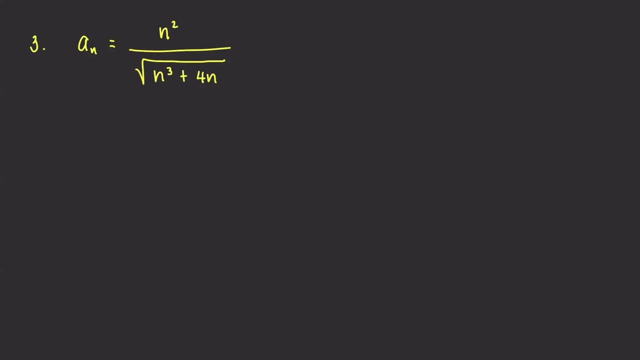 goes to infinity. it's like dividing the numerator and denominator by the highest power of n in the denominator. but since we have a radical, we also need to consider this radical here. so it's like our dominant term here is n raised to three over two square root of n cube. so that is. 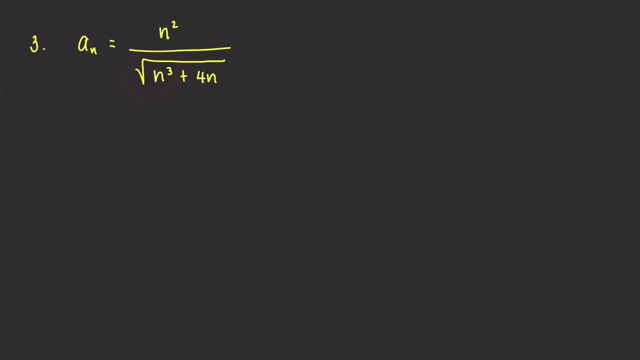 n raised to three halves. so we what we can do here is to divide the numerator and denominator by n raised to three halves, or square root of n cube. so limit of a sub n as n goes to infinity. so this is equal to limit of n squared over square root of. 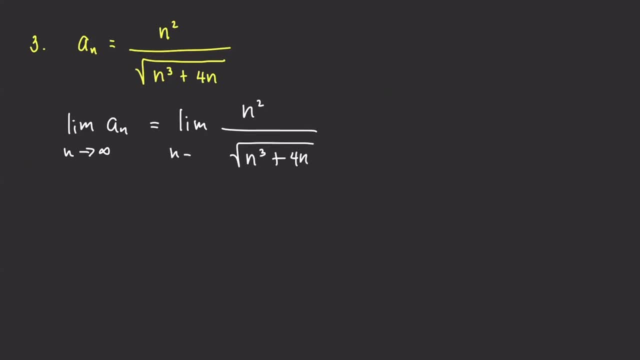 n cube plus 4n, as n goes to infinity and then we're going to. so in this case we have to multiply the numerator or divide the numerator and denominator by square root of n squared. so we'd have to have a constant minimum and we can острity the denominator by square root. 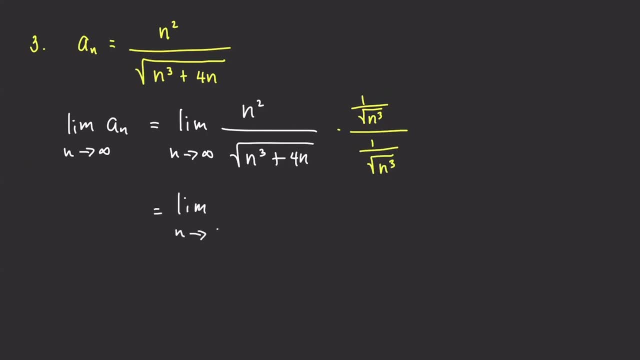 of n squared plus four over two- because we have a- is equal to n, or we can also skip this, but we can also use the number of centimeters because it's just giving. so anything is equal to 0.5 times n square root of n cubed. so what we return here is two very endpoint elements. 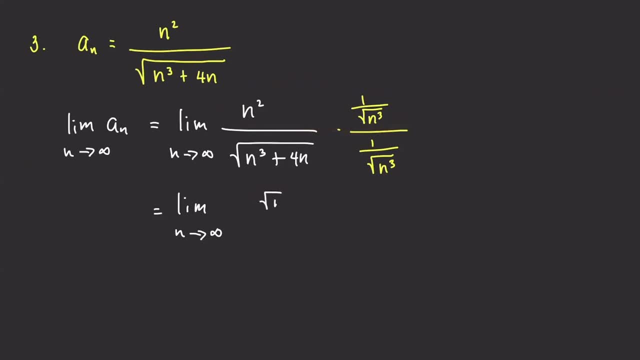 squared of n. squared of n all over, the denominator will be equal to, if we're going to write it in terms of a single radical. so you'll get here n cube plus 4n all over n cube, and this will give you limit, as n goes to infinity of squared of n all over. square root of. 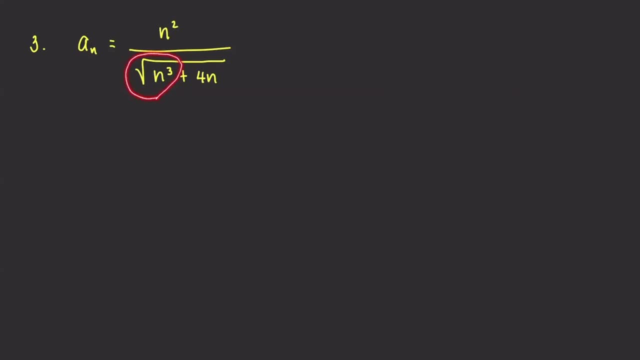 a radical. we also need to consider this radical here. so it's like our dominant term here is n. so we have n raised to three over two square root of n cube. so that is n raised to three halves. so we what we can do here is to divide the numerator and denominator by n raised to three. 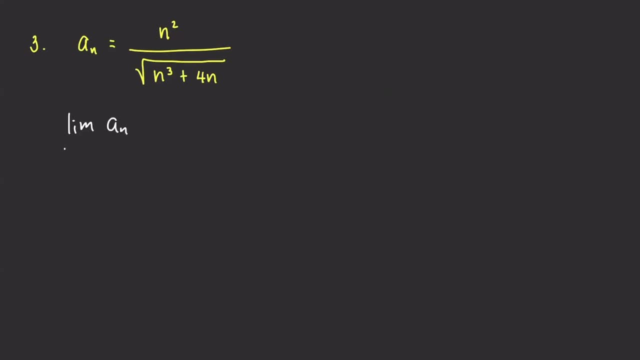 halves or square root of n cube. so limit of a sub n as n goes to infinity. so this is equal to limit of n squared over square root of n squared. so that is n raised to three halves. so that is n cubed plus four n as n goes to infinity, and then we're going to, so in this case we have to. 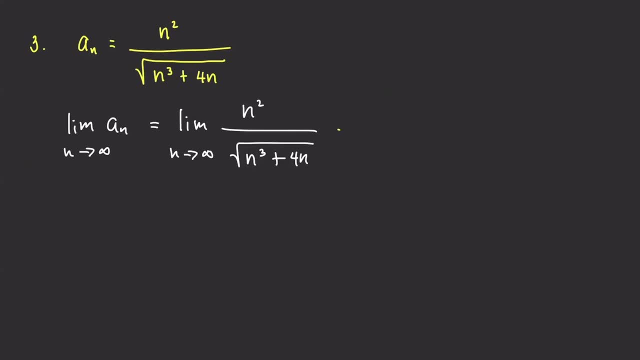 multiply the numerator or divide the numerator and denominator by square root of square root of n cube. so over one over square root of n cube, and this will give us, as n goes to infinity of n squared over n cube is equal to you have their square root of n because 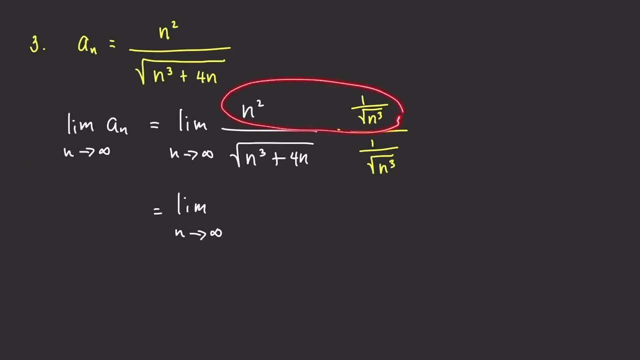 n squared is just n raised to four over two. so that will give you square root of n, square root of n. all over the denominator will be equal to. if we're going to write it into the denominator, we're going to write it into the denominator. we're going to write it into the. 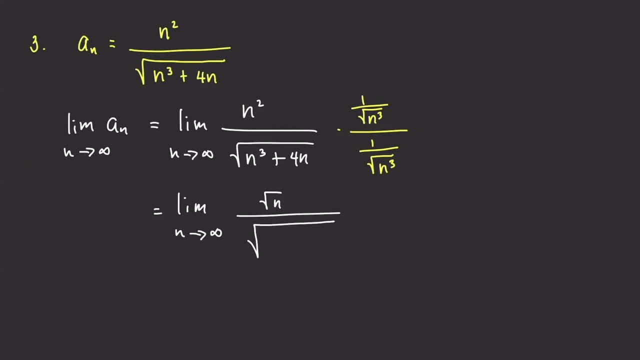 terms of a single radical. so you'll get here n cube plus four n all over n cube, and this will give you limit. as n goes to infinity of square root of n all over square root of, you have one plus four over n squared. so as n goes to infinity, so this numerator here goes to. 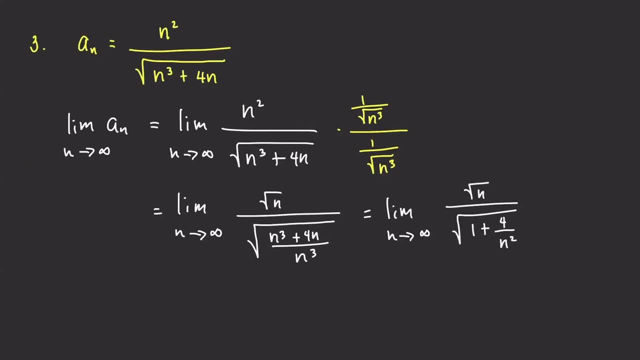 you have 1 plus 4 over n squared, so as n goes to infinity, so this numerator here goes to infinity and the denominator goes to. so this goes to 0 plus 1, it goes to 1. so it is clear from here that the limit is equal to infinity. so therefore this sequence is: 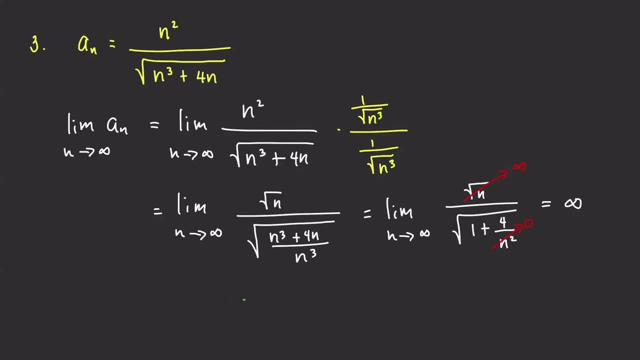 the divergent. so therefore the sequence a sub n is divergent. moving to our next problem, so we have here a sub n equal to ln of n plus 5 minus ln of n plus 2. so when we compete for the limit of a sub n, as n goes to infinity, so that is limit of this. 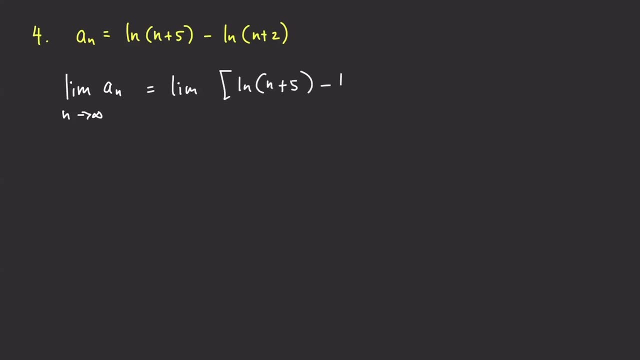 difference ln of n plus 2. so we have here a sub n equal to ln of n plus 5, minus ln of n plus 2, as n goes to infinity. so take note that the first term, this- goes to infinity, as n goes to infinity, and also the second term goes to infinity, as n goes to infinity. so that is an indeterminate form. 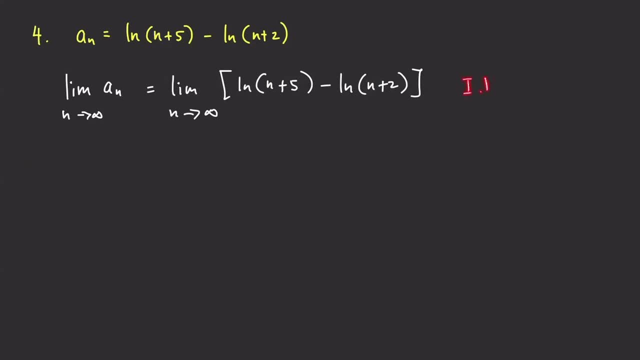 when it comes to limits, it's an indeterminate form, infinity minus infinity. and how how do we deal with such a limit? so we need to do extra work to evaluate this limit, and one way is to do some manipulation. okay, so probably here we can do, we can combine this difference into a single ln. 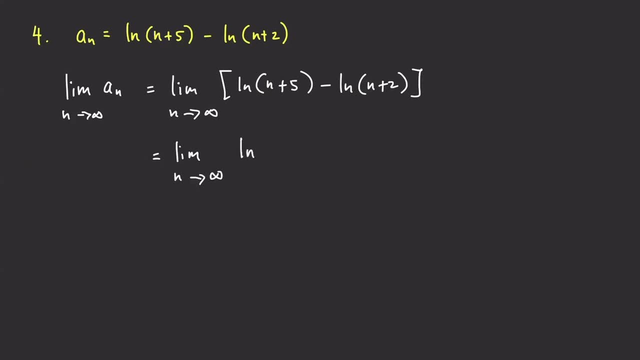 and write it down as ln of. you have here n plus 5, all over n plus 2. okay, as n goes to infinity. so take note that the second term here goes to infinity and also here we have a battie: volts of infinity. Now, what is the limit of this number inside this ln? So, as n goes to infinity, 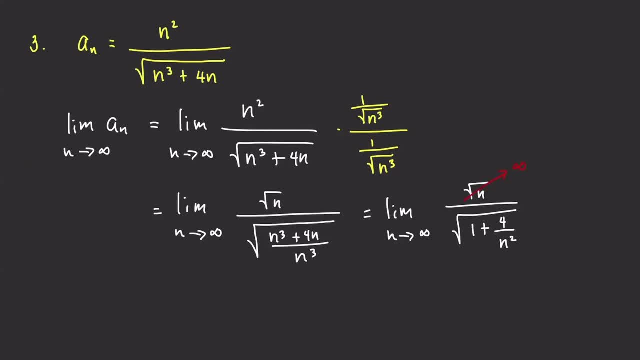 infinity and the denominator goes to. so this goes to zero plus one, it goes to one. so it is clear from here that the limit is equal to infinity. so therefore this sequence is divergent. so therefore the sequence a sub n is divergent. moving to our next problem, 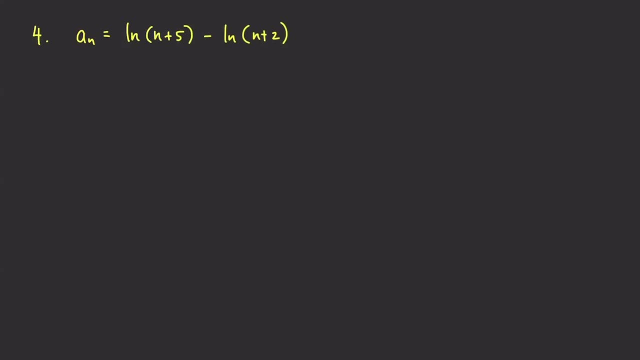 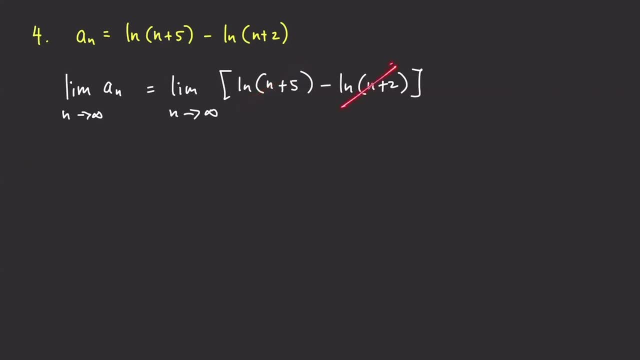 l, n of n and also the second term goes to to infinity. as n goes to infinity, so that is an indeterminate find. as n goes to infinity, so that is an indeterminate counterpart form. when it comes to limits and more complicated about the relationships between estão, defense dos al preceptores. 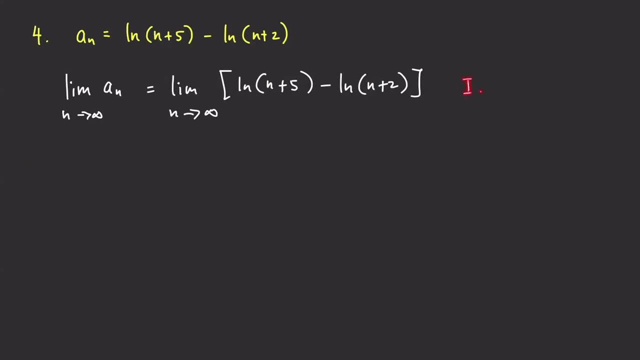 it's an indeterminate form: infinitely, as n goes to infinity. so that is an indeterminate form. when it comes to limits, it's an indeterminate form: infinity minus infinity. and how do we deal with such a limit? so we need to do extra work, is to do some. 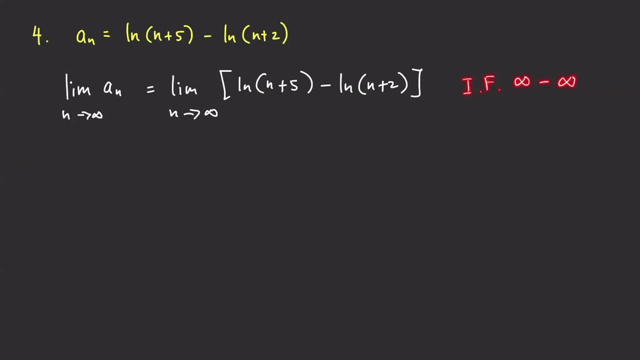 this limit, and one way is to do some manipulation. okay, so probably here we can do. we can combine this difference into a single ln and write it down as ln of. you have here n plus 5, all over n plus 2. okay, as n goes to infinity. now what is the limit of this number inside this ln? so as n. 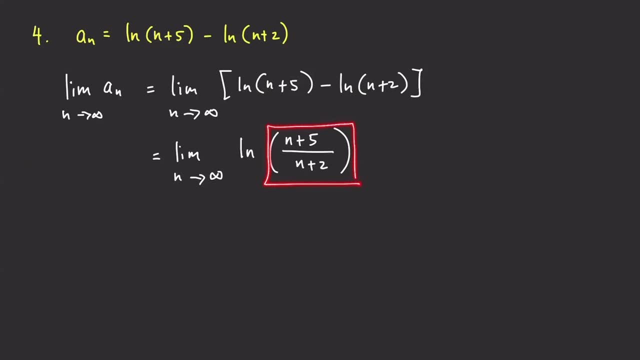 goes to infinity. we know that the limit of this one is equal to one and since ln is continuous at this limit, continuous at one, we can use a theorem which states that the limit of this is just ln of the n plus 2 limit of this expression. okay, so it's like inserting this limit inside of this ln. we can do. 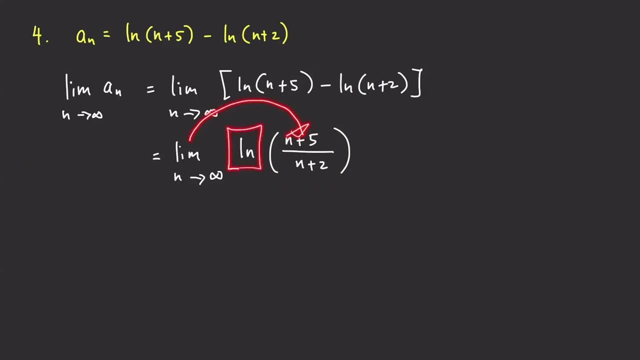 that as long as this function here is continuous, at the limit of this expression, as n goes to infinity. but we know that the limit is equal to one, so we can do that one. this is equal to a limit of ln, of the limit, as n goes to infinity, of n plus five, all over n plus two. again, keep in mind that you can only do. 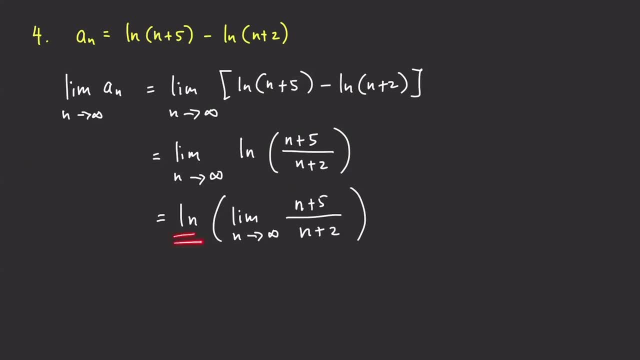 this: if this ln, ln here, okay, this function is continuous at this number, if this number exists, okay. so the limit of this one is equal to one and we can clearly see that one by expressing this fraction. of course, you can write it down: dividing the numerator and denominator by n, you'll get 1 plus 5. 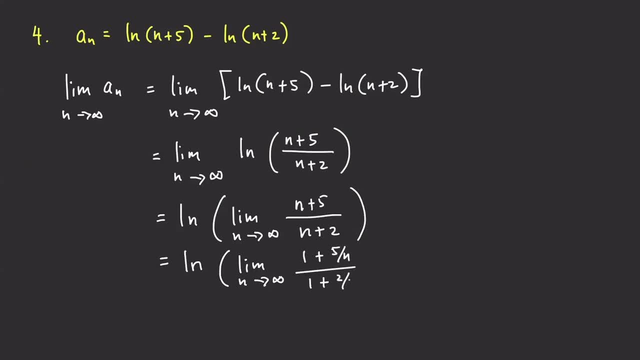 over n, all over 1 plus 2 over n. so as n goes to infinity, the numerator goes to 1, the denominator goes to 1, so this is equal to ln of 1, which is equal to 0 since the limit exists. therefore the sequence a sub n is convergent. 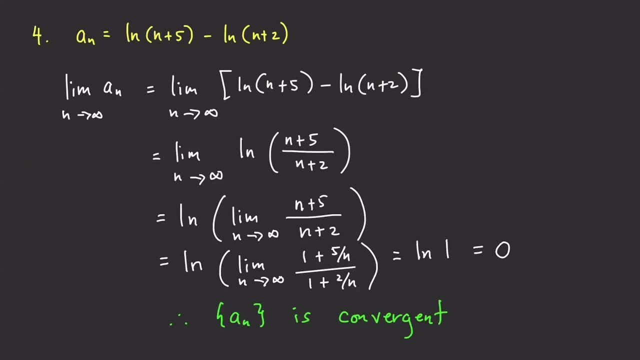 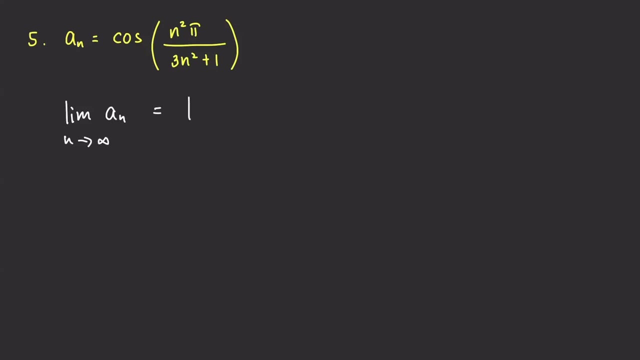 okay, next problem. so let's find the limit of this sequence here. so limit of a sub n as n goes to infinity, which is limit of cosine of n squared times pi all over 3n squared plus 1, as n goes to infinity. so the, this cosine function is continuous everywhere. all right, so as long as the limit of this expression. 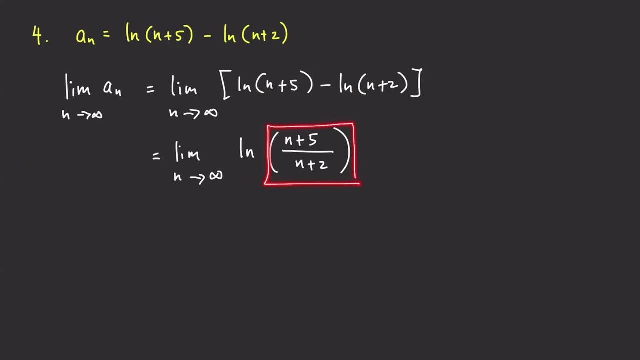 we know that the limit of this one is equal to one, And since ln is continuous at this limit, continuous at one, we can use a theorem which states that the limit of this is just the ln of the limit of this expression. Okay, So it's like inserting this limit inside of 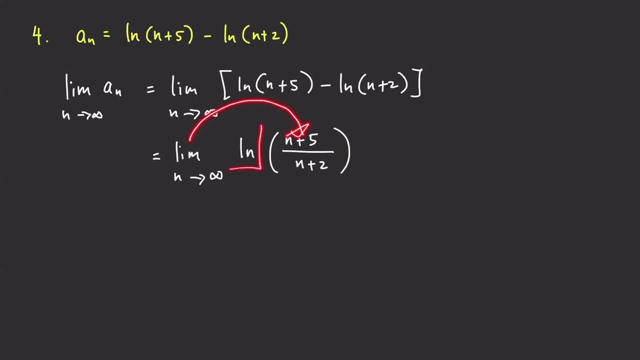 this ln. We can do that as long as this function here is continuous, at the limit of this expression, as n goes to infinity. But we know that the limit is equal to one, So we can do that one. This is equal to limit of ln. 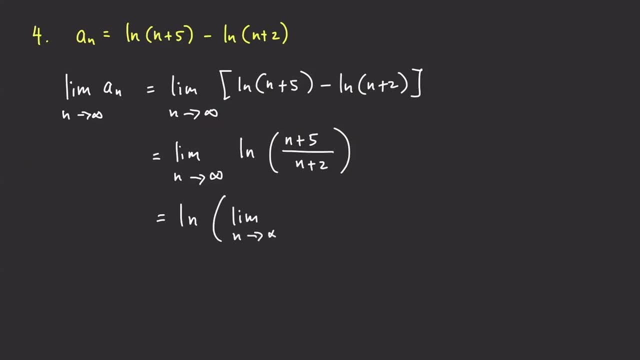 The limit, as n goes to infinity, of n plus five, all over n plus two. Again, keep in mind that you can only do this if this ln here. okay, this function is continuous at this number, if this number exists. Okay. So the limit of this one is equal to one, and we can clearly see that. 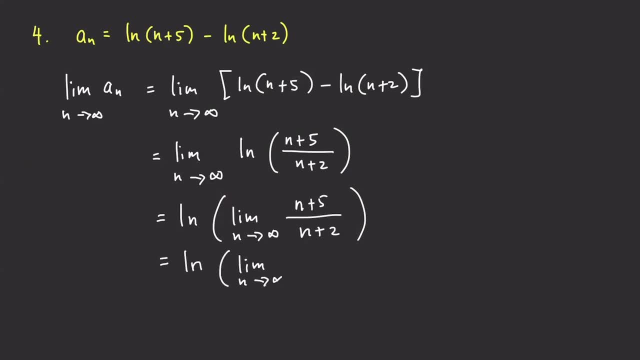 one by expression. So if we keep pressing this fraction, of course you can write it down Dividing the numerator and denominator by n, you'll get one plus five over n, all over one plus two over n. So as n goes to infinity, the numerator goes to one, the denominator goes to one, So this: 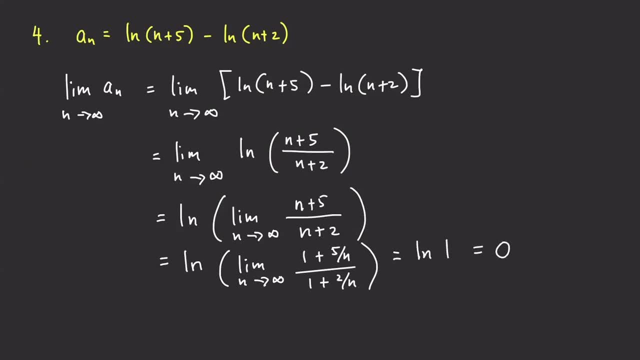 is equal to ln of one, which is equal to zero. Since the limit exists, therefore, the sequence a sub n is convergent. Okay, next problem. So let's find the limit of this sequence here. So limit of a sub n, as n goes to infinity. 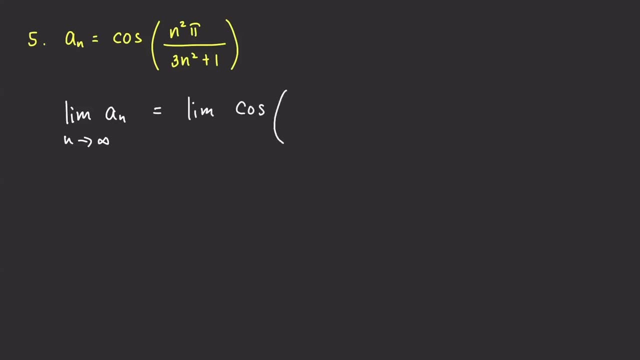 which is limit of cosine of n squared times pi, all over three n squared plus one as n goes to infinity. So this cosine function is continuous everywhere. All right. So as long as the limit of this expression exists, then we can insert this limit here, And the limit of this one is just the cosine. 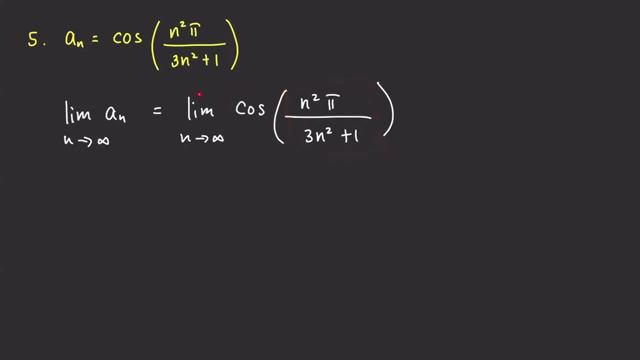 exists, then we can insert this limit here. and the limit of this one is just the cosine of the limit of this expression. okay, and what is the limit of that one? if you look at this expression here, we know that the limit of this is equal to one-third. okay, because when you're looking for 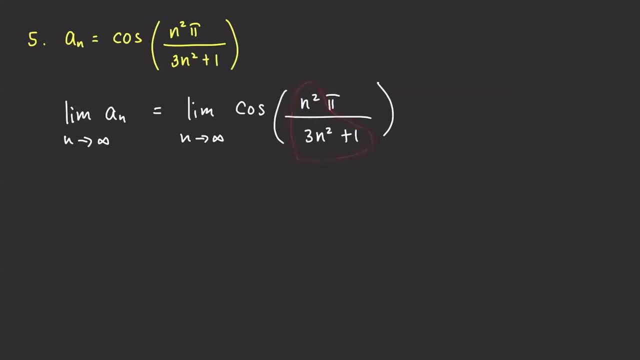 limit at infinity. you're actually looking for the limit of the dominant term in the numerator and dominant term in the denominator. you have this one here and this one goes to pi over three as n goes to infinity. so the limit of that one we can write it down as a cosine. 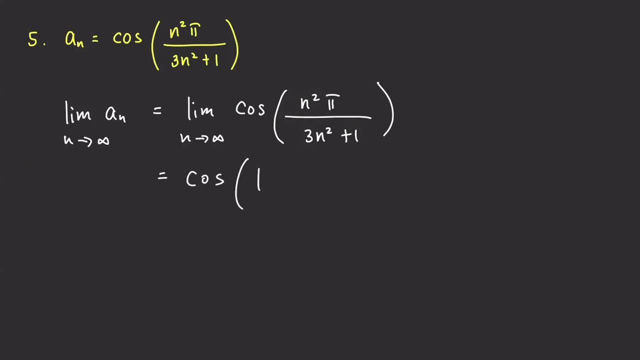 of the limit, as n goes to infinity of this expression here, and what i can, what we'll do now is to divide the numerator and denominator by n squared, and that will give you pi over three plus one over n squared. okay, so that is multiplying the numerator and denominator. 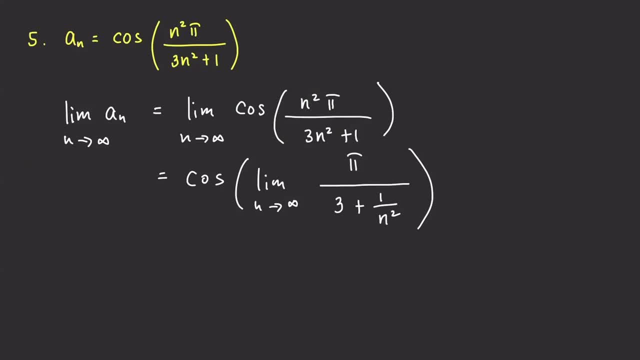 by one over n squared, which is the same thing as dividing the numerator and denominator by n squared. and from here it is clear that the limit of this denominator here is equal to three, because this goes to zero. so therefore this is equal to the cosine of pi over three, and 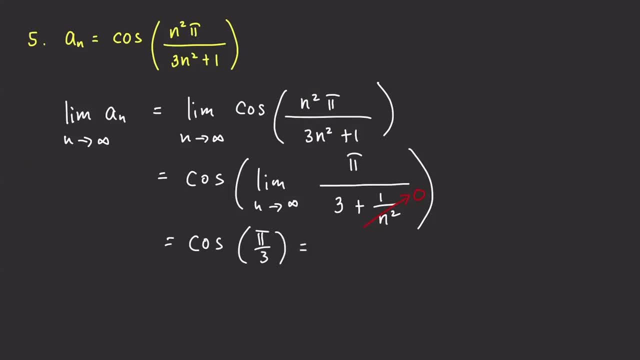 what is cosine of pi over three? It is equal to one-half. since the limit exists, this sequence, a sub n, is convergent. next let's look at this sequence here, which is a sub n equal to n, factorial over to n. so how do we find this, the limit of this sequence? so here we're going to try to apply. 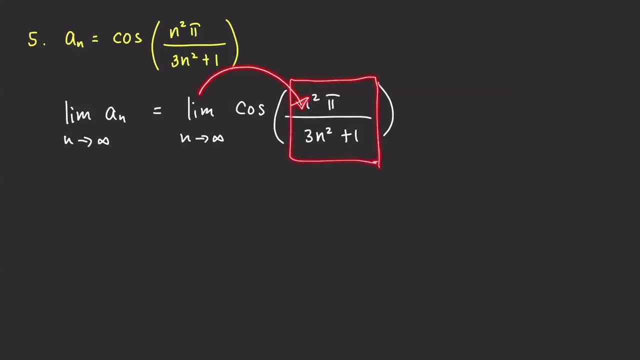 of the limit of this expression. Okay, And what is the limit of that one? If you look at this expression here, we know that the limit of this is equal to one third, So we can write it down as a cosine of the limit of this expression. Okay, Because when you're 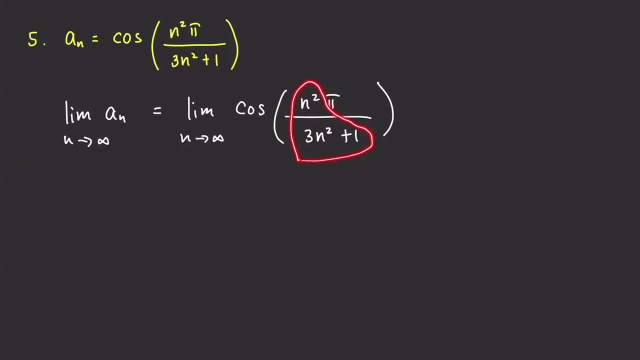 looking for limit at infinity. you're actually looking for the limit of the dominant term in the numerator and dominant term in the denominator. You have this one here And this one goes to pi over three as n goes to infinity. So the limit of that one we can write it. 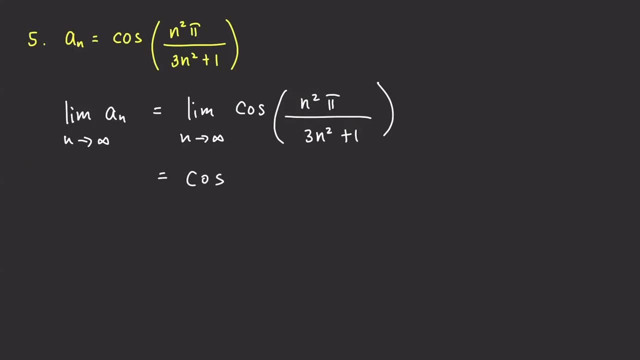 down as a cosine of the limit. And then from here we have this: So this is a cosine of the limit, as n goes to infinity, and that'll give us pi over three plus one over n squared. Okay, So that is multiplying the numerator and denominator by one over n squared, which is the same as the denominator. of the denominator. Okay, So we're gonna leave that with a p And then we're gonna write that down like this: Okay, So, right here we're gonna write that down. So we're gonna add a number to the numerator. 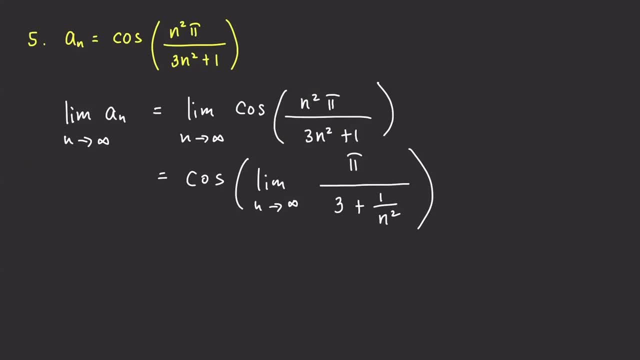 So we're gonna divide by n squared and that will give us pi over three plus one over n squared thing as dividing the numerator and denominator by n squared. And from here it is clear that the limit of this denominator here is equal to three, because this goes to zero. So therefore, 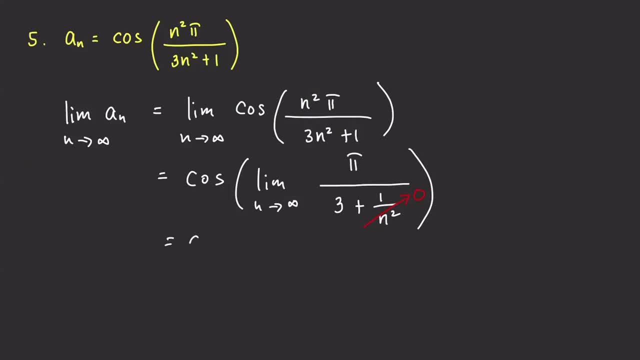 this is equal to the cosine of pi over three. And what is cosine of pi over three? It is equal to one half. Since the limit exists, this sequence, a sub n, is convergent. Next, let's look at this sequence here, which is a sub n equal to n. factorial over n raised to n. 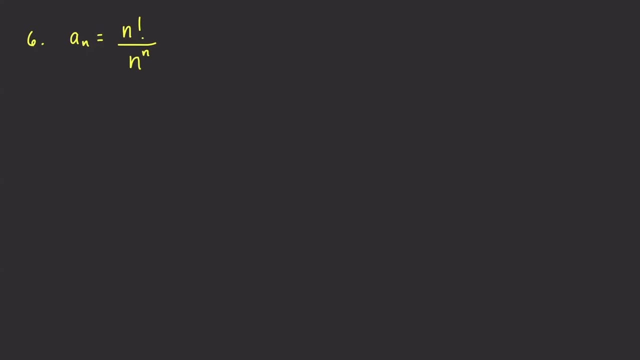 So how do we find that? So how do we find the limit of this sequence? So here we're going to try to apply this squeeze theorem. So take note that this n, factorial over n, raised to n here is, of course it is greater than or equal to zero. So we're assuming here that our n is greater than or equal. 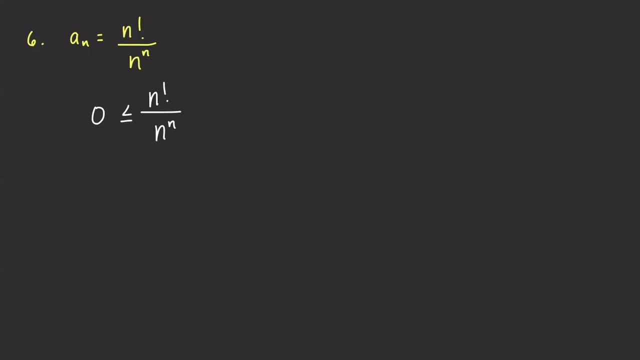 to one. So you have there greater than or equal to zero, But actually n factorial, by definition, is n times. you have there n minus one, and then you have times n minus two. OK, So let me write this one as like this: OK, N minus one times, n minus two times, and so on. 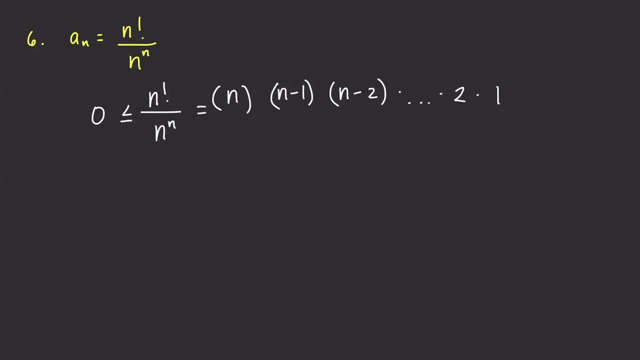 times two and then times one and the n raised to n. so it's like we have n copies of n. so let's write that down as something like this: over n over n, okay, and then over n and so on, okay. so you have here over n and then over n. 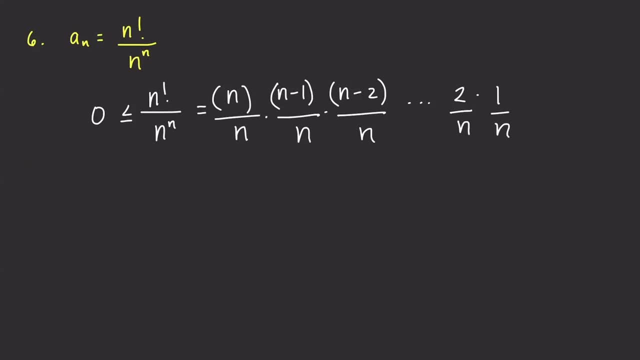 so, as you can see from this one, so the product of our denominators are just equal to n raised to n, and of course the product of all the numerators here is equal to n- factorial. now, since we're planning to use a squeeze theorem, if we look at these expressions here, 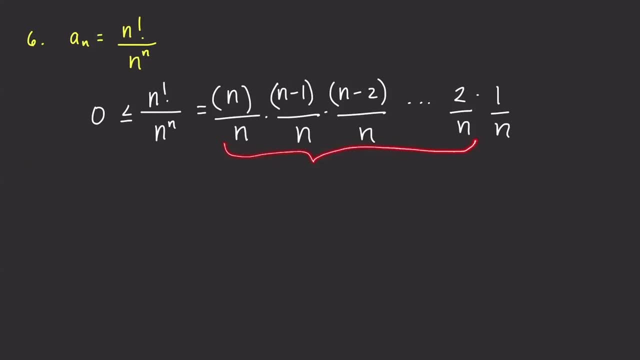 okay. the numerator is always less than or equal to the denominator. so therefore we have the numerator, and the numerator is always less than or equal to the denominator. so therefore we have, in this case, this is always less than or equal to one. it's actually equal to one, this one, it is strictly less than one. 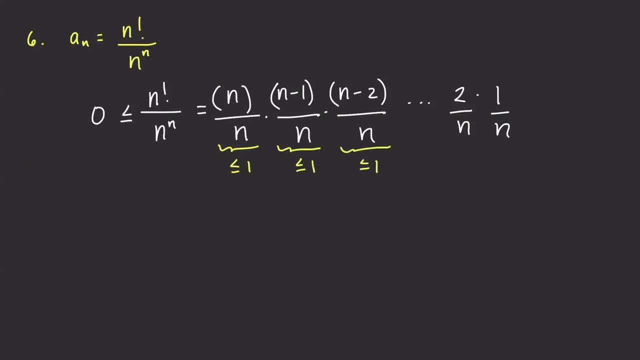 but i can also write it as less than or equal to one, and so on. up to this one, it is less than or equal to one. okay, for n greater than or equal to two, all right. so if n is equal to one, of course we only get one over n. 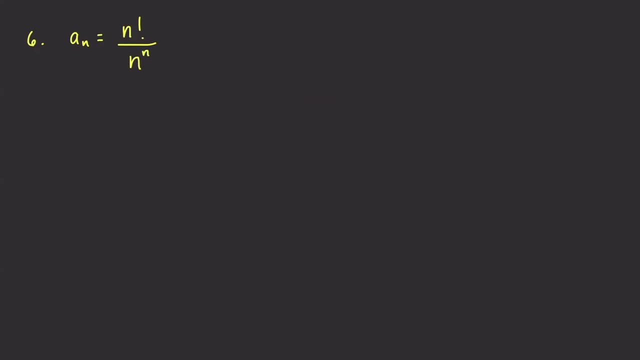 squeeze theorem. so take note that this n factorial over n raised to n here. okay is of course it is greater than or equal to zero. so we're assuming here that our n is, uh, greater than or equal to one. okay, so you have there greater than or equal to zero, but actually 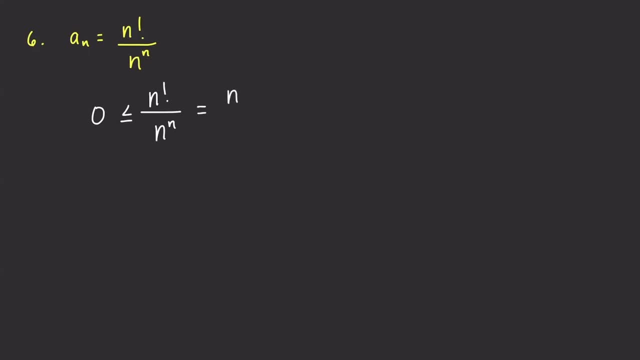 n. factorial, by definition, is n times. you have there n minus 1, and then you have times n minus 2. okay, so let me write this one as like this: okay, n minus 1 times, n minus 2 times, and so on times 2 and then times 1.. and the n raised to n. so it's like we have n copies of n. so let's write that: 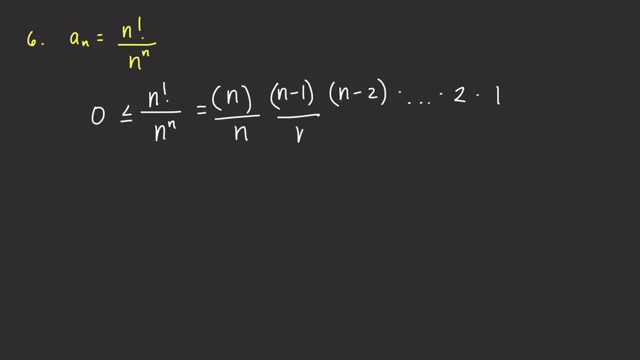 down as something like this: over n, over n, okay, and then over n and so on, okay, so you have here over n and then over n. so as you can see from this one, so the product of our denominators are just equal to n raised to n and of course the product of all the numerators here is equal to. 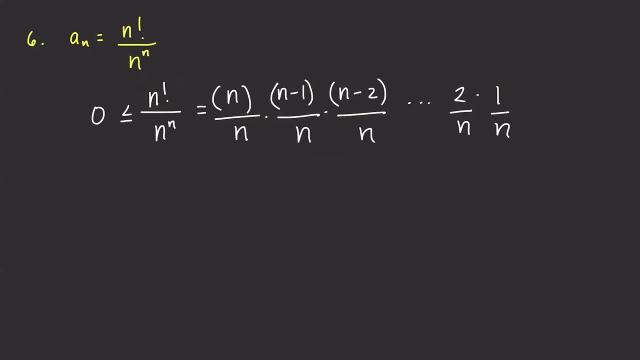 n factorial. now, since we're planning to use a squeeze theorem, if we look at these expressions here, okay, the numerator is always less than or equal to the denominator, so therefore we have: in this case, this is always less than or equal to one. it's actually equal to one. 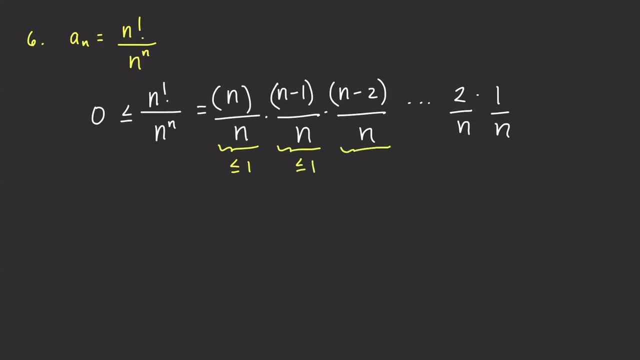 this one, it is strictly less than one, but i can also write it as less than or equal to one, and so on. up to this one, it is less than or equal to one. okay, for n greater than or equal to two, all right. so if n is equal to one, of course we only get one over n. 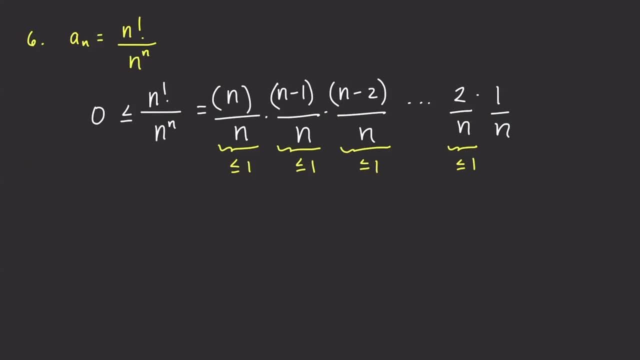 okay. so in this case we can use an upper bound, the function, okay, or the sequence, one over n: okay. so we have here a factor. this factor here is just less than or equal to one. you're just multiplying positive numbers that are less than or equal to one, so you would expect that the product 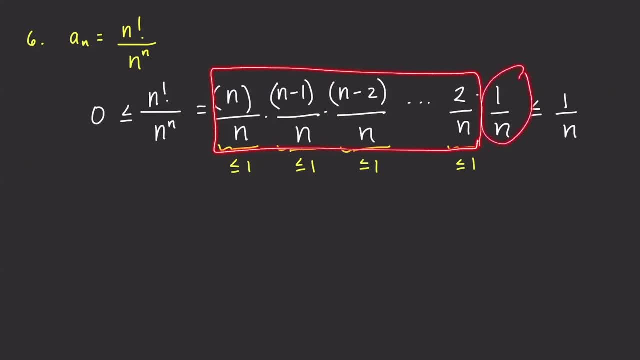 is less than or equal to one. so when you multiply that by one over n, the product will be less than or equal to one over n. so if we let this function here to be our b sub n and this, uh, okay, it's like you have a sequence of. 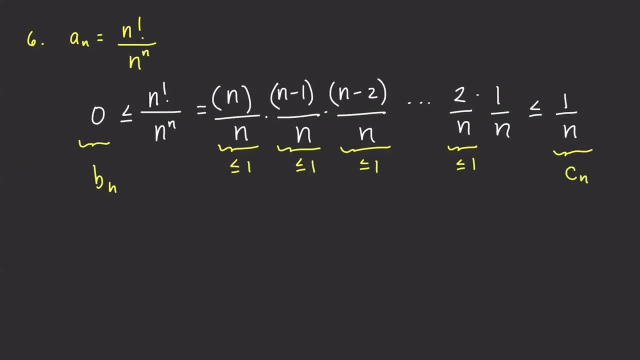 zeros. okay, and then another sequence here: c sub n, which is equal to one over n for any n. so since, since, uh, the limit of b sub n, or, let's write it down first, okay, so since in this case your b sub n is less than or equal to your a sub n, which is less than or equal to c sub n. 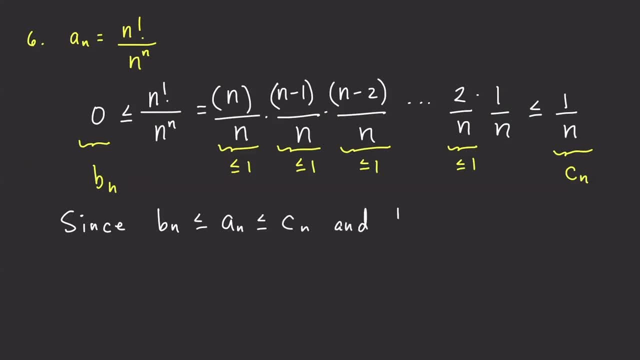 and in this case the limit of b sub n as n goes to infinity is equal to 0, which is also the same thing as the limit of the c sub n as n goes to infinity. so by squeeze theorem or sandwich theorem, so by squeeze theorem, we can conclude that the limit of a sub n as n goes to infinity is equal to zero. 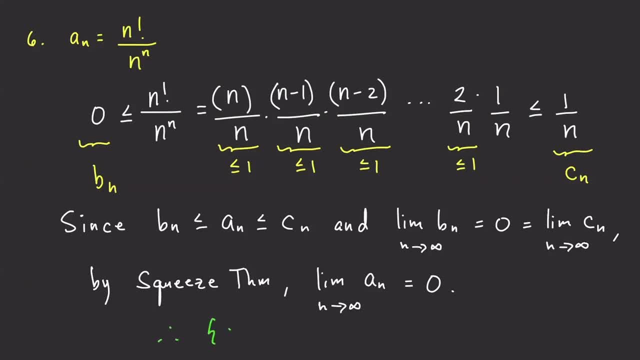 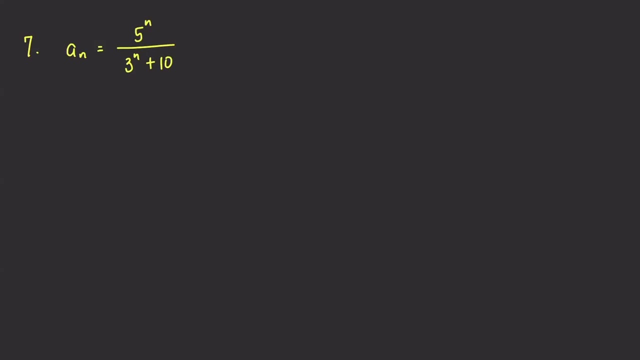 since the limit exists, we can conclude that the sequence a sub n is convergent. so we can conclude that the sequence a sub n is convergent. next problem. so now let's look at this one here. so we're given a sub n equal to 5 raised to n over a 3 raised to n plus 10.. again, same as the technique that 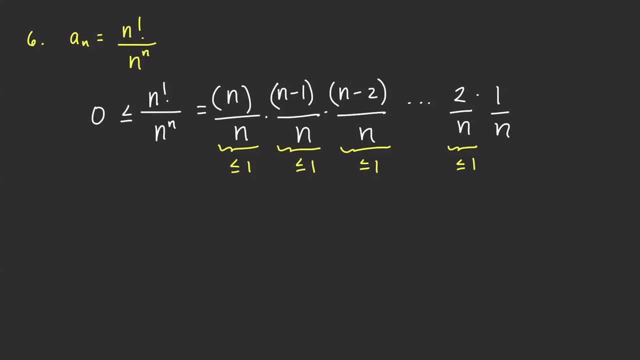 okay, so and so on. up to this one. we can also write this on. up to this one here. so in this case we can use an upper bound, the function okay, or the sequence one over n: okay. so we have here a factor. this factory here is just less than or equal to one. you're just multiplying positive. 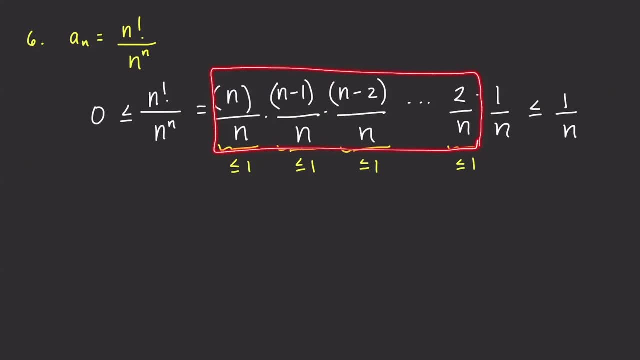 numbers that are less than or equal to one. so you would expect that the product by 1 over n, the product will be less than or equal to 1 over n. so if we let this function here to be our B sub n and this, okay, it's like you have a sequence. 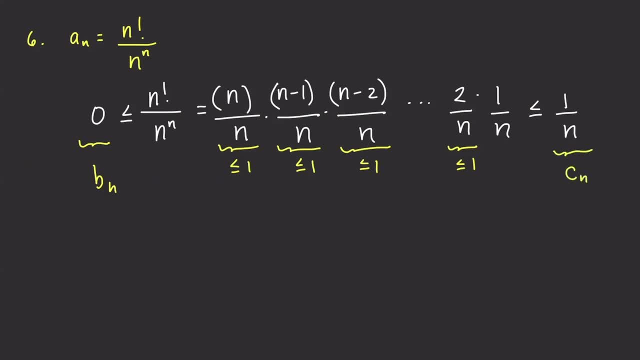 of zeros. okay, and then another sequence here: C sub n, which is equal to 1 over n for any n. so since, since, limit of B sub n, or let's write it down first, okay, so since in this case your B sub n is less than or equal to your a sub n, which is 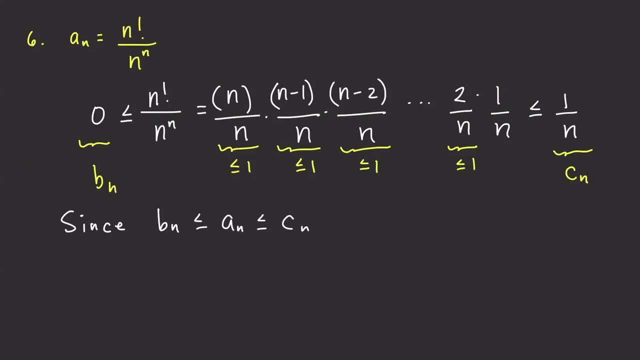 less than or equal to C sub n, and in this case the limit of B sub n, as n goes to infinity, is equal to zero, which is also the same thing as the limit of the C sub n, as n goes to infinity. so by squeeze theorem, or sandwich theorem, so by squeeze theorem, we can conclude that the limit 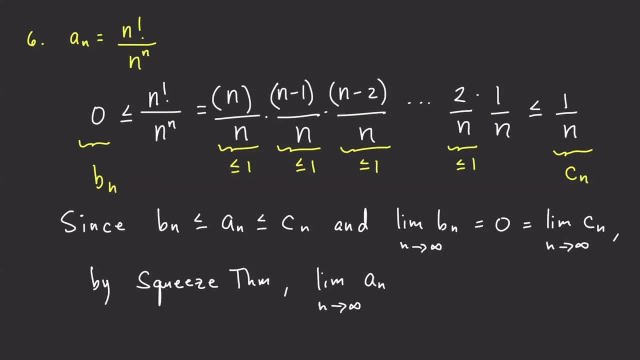 of a sub n, as n goes to infinity, is equal to zero, since, Since the limit exists, we can conclude that the sequence a sub n is convergent. Next problem. So now let's look at this one here. So we're given a sub n equal to 5 raised to n over 3, raised to n plus 10.. 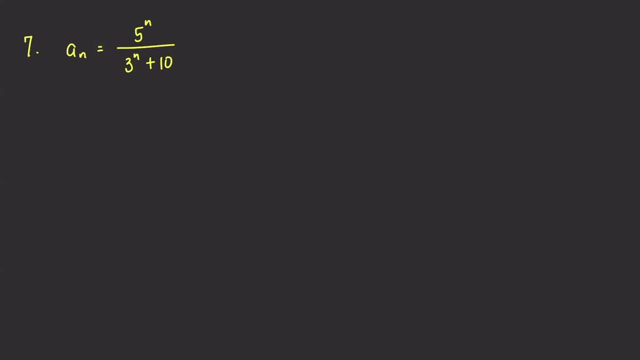 Again same as the technique that we've been using to evaluate limit of rational functions. This is your dominant term in the denominator. So we divide the numerator and denominator by this dominant term. So we compute for limit of a sub n, as n goes to infinity. 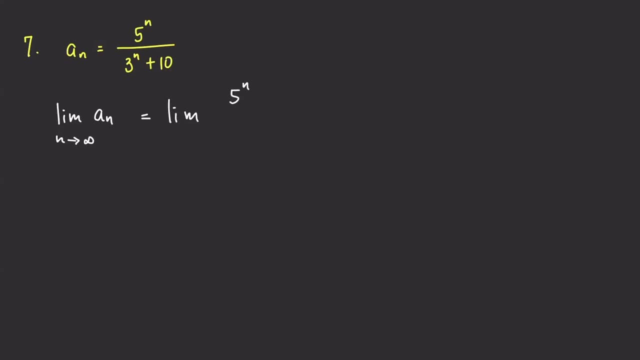 which is equal to limit of 5 raised to n, 3 raised to n plus 10, as n goes to infinity, And dividing the numerator and denominator by 3 raised to n. So we have here dividing the numerator and denominator by 3 raised to n. 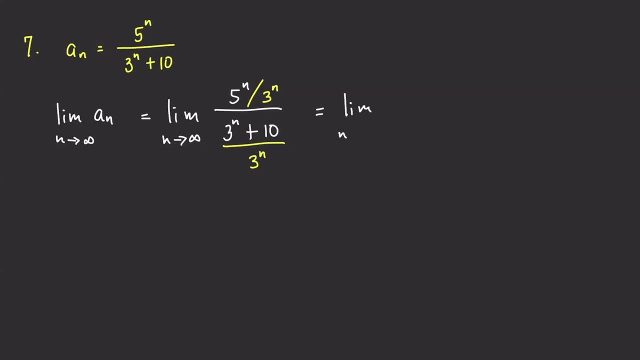 we'll get limit as n goes to infinity of you have here 5 over 3 to the n over. you have here 1 plus 10 over 3 raised to n. Now, since this base here is greater than 1,, 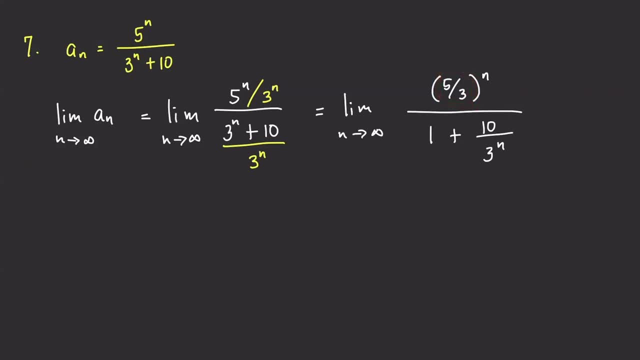 we know that this numerator goes to what? Okay, it goes to infinity, as n goes to infinity. Now, this term in the denominator goes to 0, as n goes to infinity. So therefore, the limit is equal to infinity, Since it's infinity. 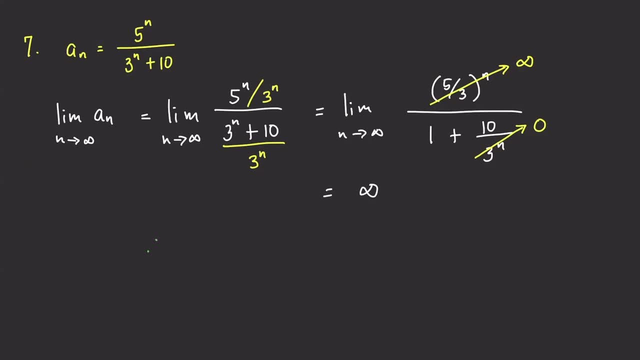 it's not a. it's not a real number. we conclude that the sequence a sub n is divergent, Moving to our last problem here. So let's determine whether this sequence here is convergent or divergent. Okay, let's now move to our last problem. 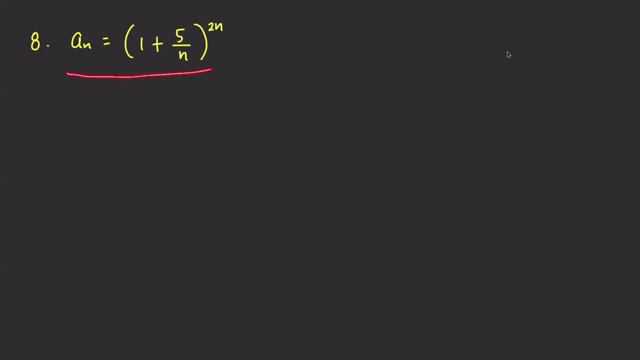 So let's determine whether this sequence is convergent or divergent. So again, we compute for limit of a sub n as n goes to infinity, which is equal to limit of 1 plus 5 over n raised to 2n, as n goes to infinity. 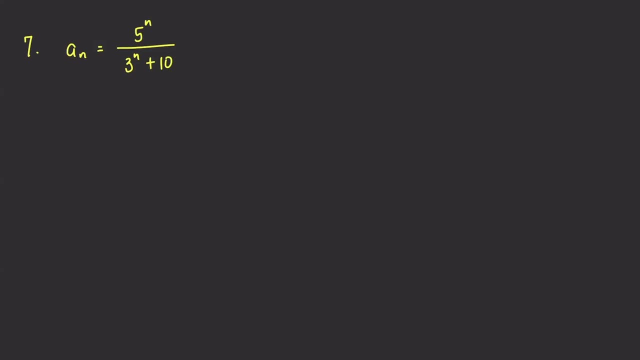 we've been using to evaluate limit of rational functions. this is your dominant term in the denominator. so we divide the numerator and denominator by this dominant term. so we compute for limit of a sub n, as n goes to infinity, which is equal to limit of 5 raised to n. 3 raised to n plus 10, as n goes to infinity. and dividing the numerator and denominator, 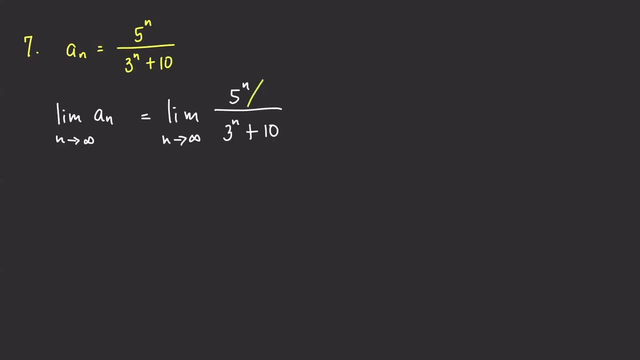 by uh, 3 raised to n. okay, so we have here dividing the numerator and the denominator by 2 raised to n, we'll get limit as n goes to infinity of you have here 5 over 3 to the n over. you have here 1 plus 10 over 3 raised to n. 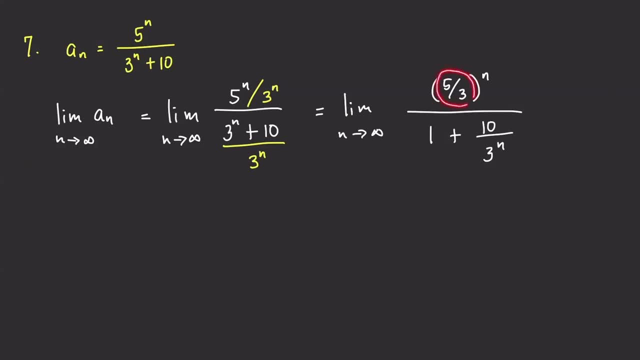 now, since this base here is greater than 1, we know that this numerator goes to what. okay, it goes to infinity, as n goes to infinity. now, uh, this term in the denominator goes to zero, as n goes to infinity. so therefore, the limit is equal to infinity, since it's infinity, it's. 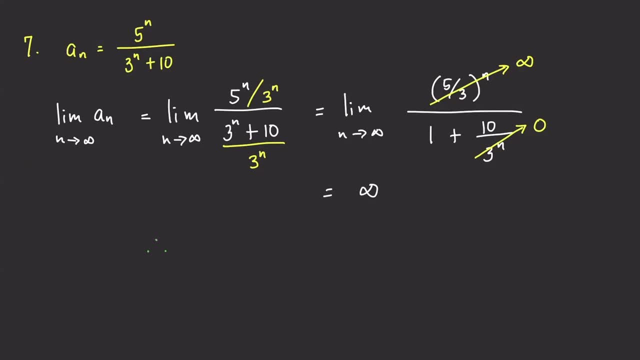 not a real number. we conclude that the sequence a sub n is divergent. okay, so now let's move on to our last problem. moving to our last problem here, so let's determine whether this sequence here is convergent or divergent. okay, let's now move to our last problem. so let's determine whether this sequence is convergent or. 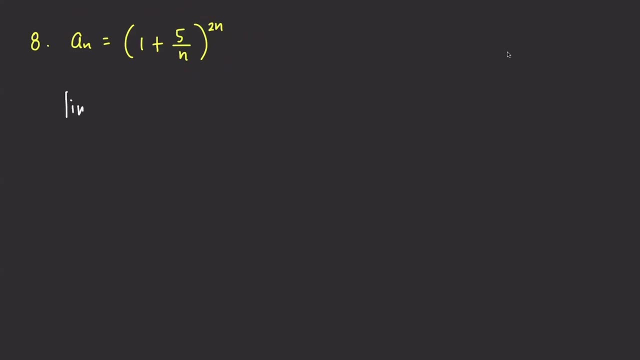 so again we compute for limit of a sub n as n goes to infinity, which is equal to limit of 1 plus 5 over n raised to 2n, as n goes to infinity. okay, so if we look at this one, the base here, as n goes to infinity, it goes to 1, and the power or the 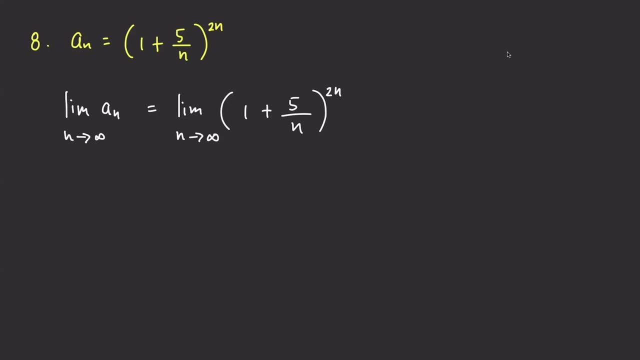 Okay. so if we look at this one, the base here, as n goes to infinity, it goes to 1 and the power or the exponent goes to infinity as n goes to infinity. So the limit here is in the form: 1 raised to infinity. 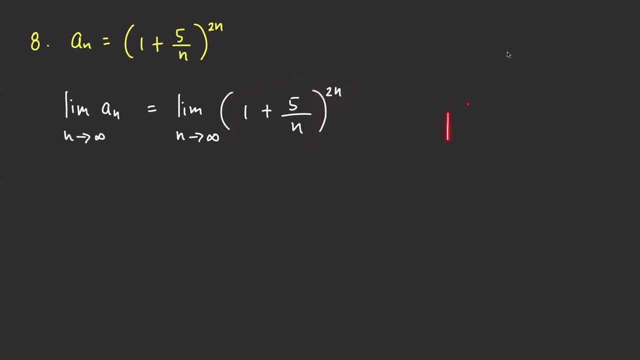 which is actually one of the indeterminate forms. If you have a limit, something like this, it is an indeterminate form. So you may apply here El-Hopital's rule. but I think to easily evaluate the limit you just have to recall the definition of e. 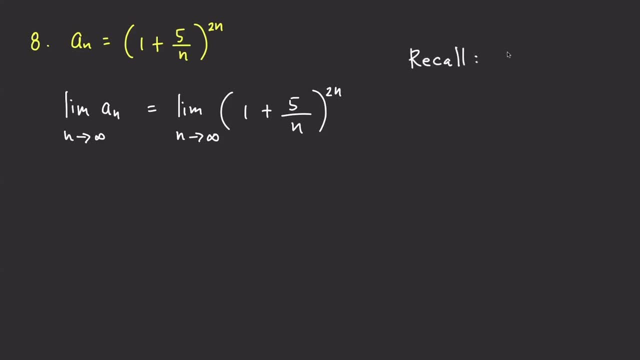 So what is one way to define the number e? So the number e, this irrational number, real number e is defined to be the limit of 1 plus 1 over m, raised to m, as m goes to infinity. So that is one way to define this number e. 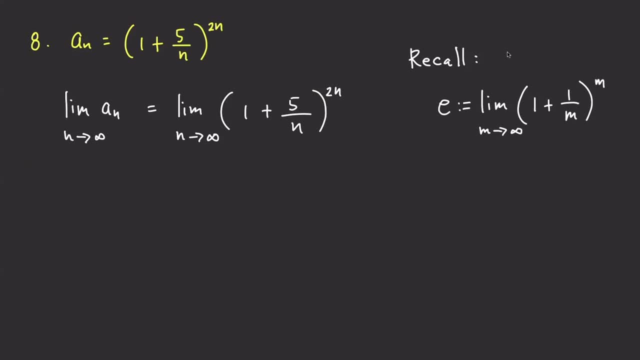 It's the limit of this expression, as m goes to infinity. So if we know this fact, so we can easily compute for the limit of this sequence, So we may write it as limit, as n goes to infinity. of you have here 1 plus. 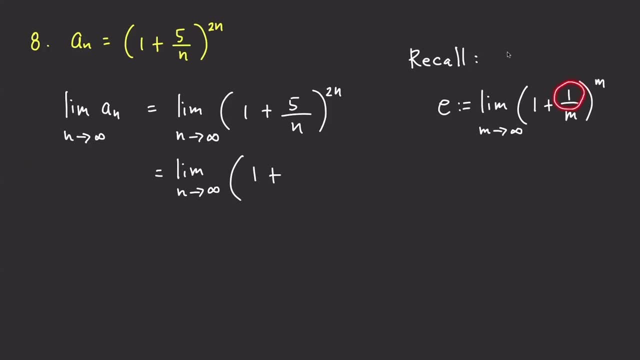 we want to look at this. we want this to look like this. It should be 1 over m, So we need to write this 5 over n as 1 over n over 5.. Okay, And we can write our numerator as: 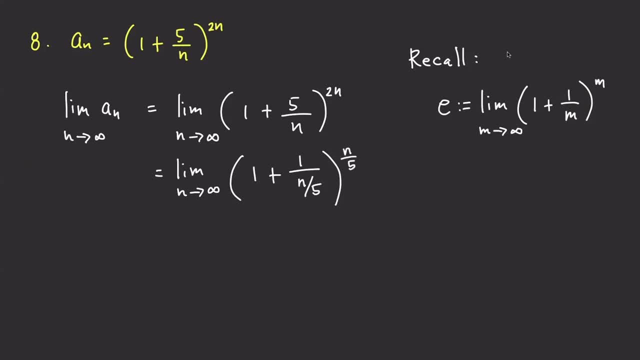 we need to produce n over 5 here, But since the power is 2n, so we need to multiply this n over 5 by, of course, in this case by 10. So that when you take the product, it's equal to 2n. 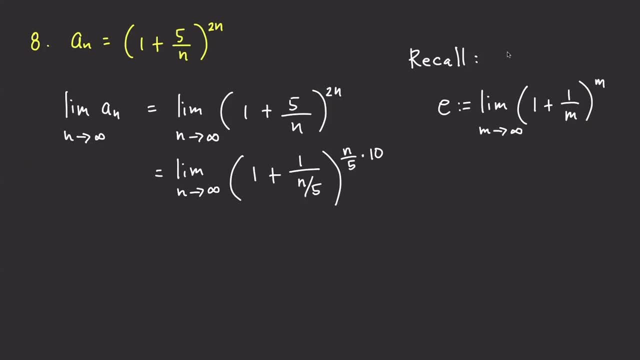 So now we can write this down as limit, as m goes to infinity. So we're going to have a change of variable here: 1 plus 1 over m, 1 plus 1 over m, 1 plus 1 over m. 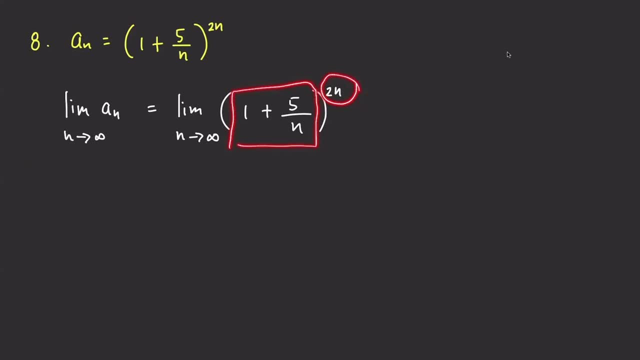 component goes to infinity, as n goes to infinity. so the limit here is in the form 1 raised to infinity, which is actually one of the indeterminate forms. if you have a limit, something like this, it is an indeterminate form. so you may apply here el hopital's rule. but 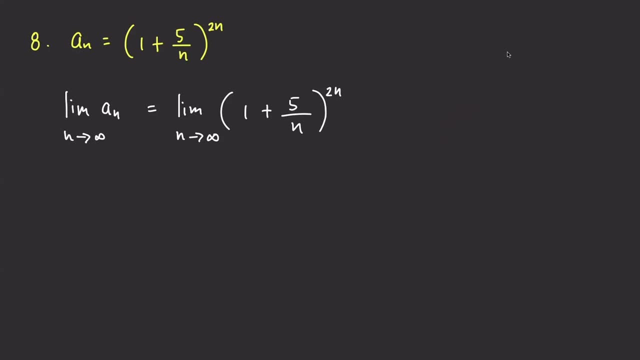 i think to easily evaluate the limit, you just have to recall the definition of e. so what is one way to define the number e? so the number e is this irrational number, okay, real number, okay. e is defined to be the limit of 1 plus 1 over m raised to m, as m goes to infinity. so that is one way to define this number. 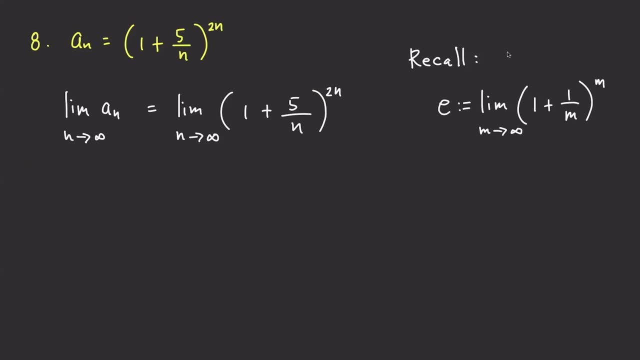 E, it's the one way limit of this expression, as m goes to infinity. so if we know this effect, so we can easily compete for the limit of this sequence, so we may write it as limit, as n goes to infinity, of you have here 1. 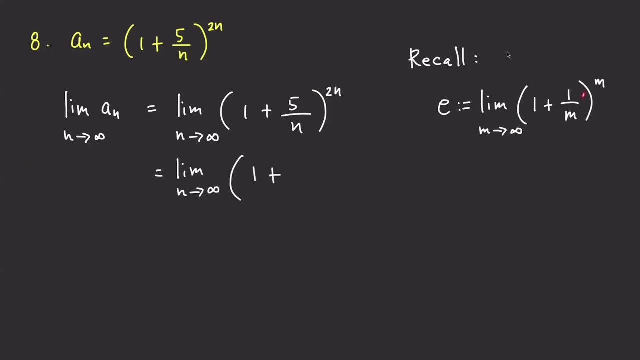 plus, we want to look, uh at this. we want this to look like this. it should be 1 over m, so we need to write this 5 over n as 1 over n over 5. okay, and we can write our numerator as we need to produce. 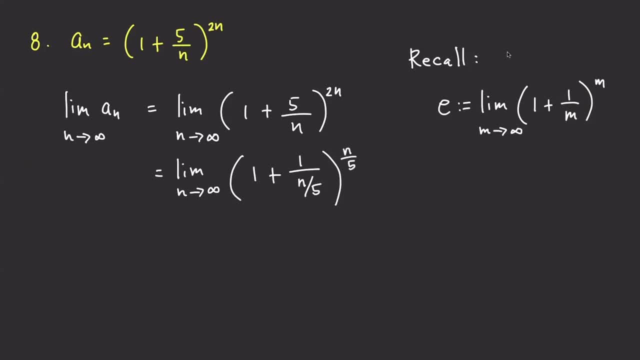 n over 5 here, but since the power is 2n, so we need to multiply this n over 5 by, of course, in this case by 10, so that when you take the product it's equal to 2n. so now we can write this down as limit, as m goes to infinity. so we're going. 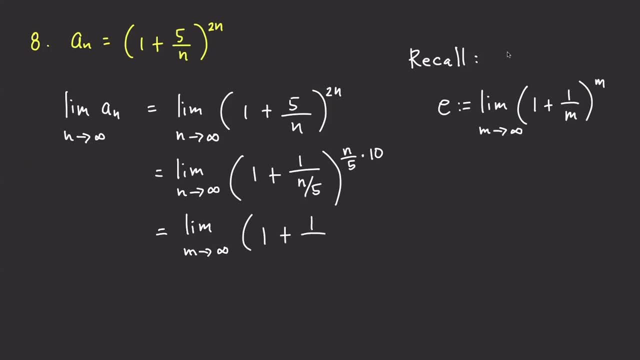 to have a change of variable here: 1 plus 1 over m, raised to m times 10. okay, but rule on exponents. i can actually write this down as this expression and then quantity raised to 10.. what is the m here? m is equal to n over 5, and take note that as n goes to infinity, 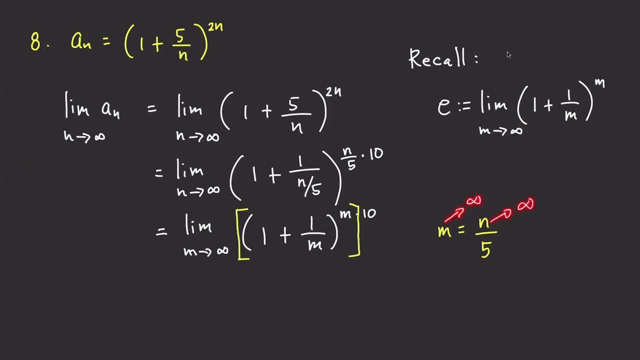 this m here also goes to infinity. so now, since we know that the limit of this expression, as m goes to infinity, is equal to e, so therefore this limit is just e raise to 10, and since this is just a real number, we can conclude that the sequence a sub n is convergent. so for you to easily evaluate this, for example the limit. 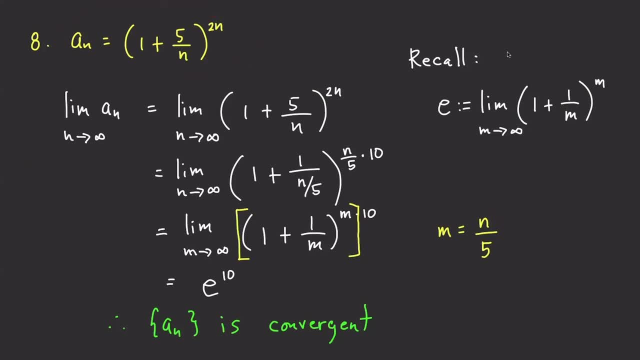 of this kind of expression. so it is helpful to remember that the limit of, let's say, 1 plus a over n- okay, so let me write this as a over n and then raised to n, as n goes to infinity- is just equal to e raised to a. and this is true for this is for any a, any real number, a. so if you know this fact, okay, 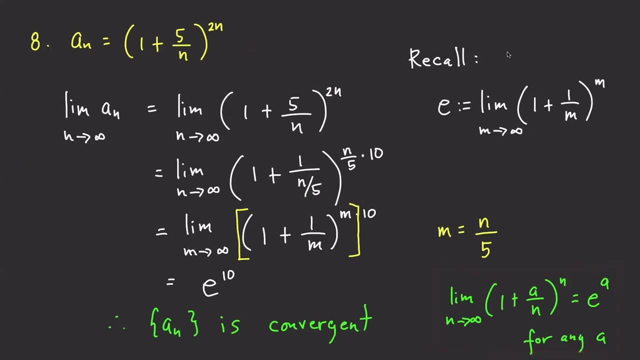 you can easily evaluate this one here, because you can just compute for this limit here. okay, without the 2, and the limit of that one is just equal to e raised to 5, and then, of course, quantity squared, you'll get a limit of that one, and then, of course, quantity squared, you'll get e raised to a, and then 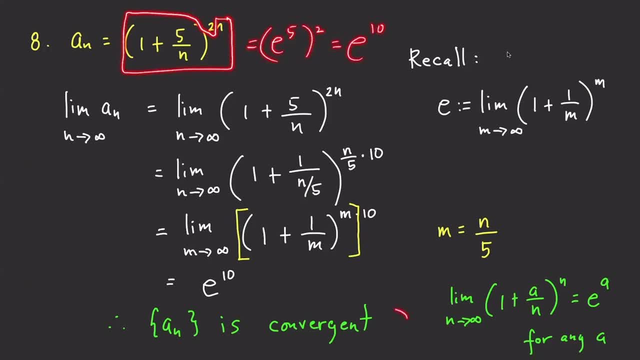 get e raised to 10.. So therefore, you can conclude immediately that your sequence is convergent.